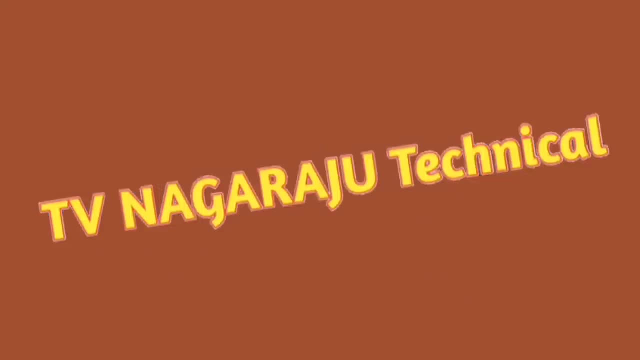 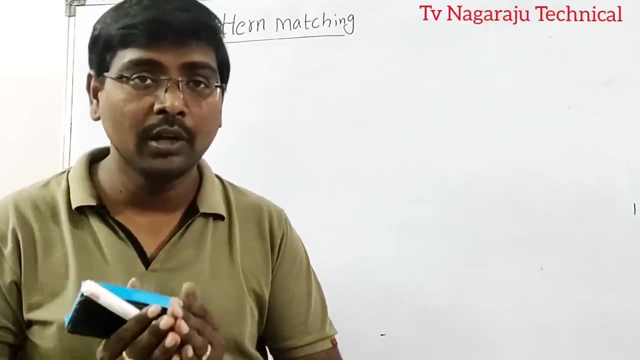 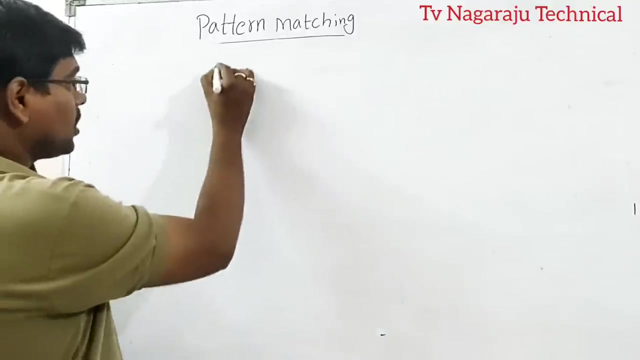 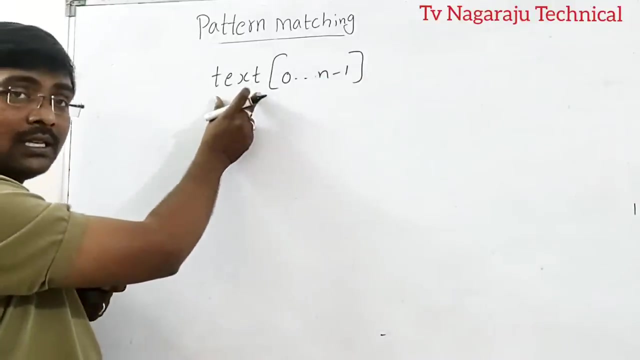 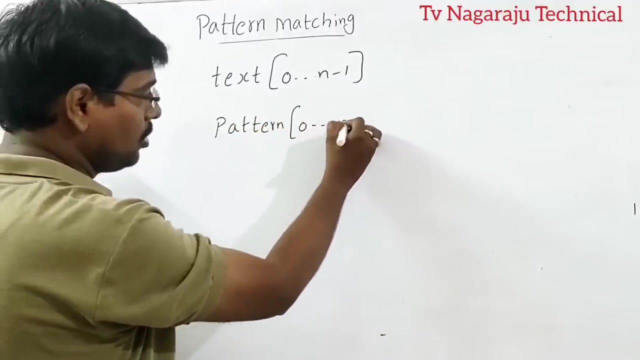 Welcome to our channel. In this session we are going to discuss about pattern matching. What is mean by pattern matching? Consider two strings, For example. my first string is text of 0 to n-1.. This is a string of length n. and consider one more string, pattern 0 to. 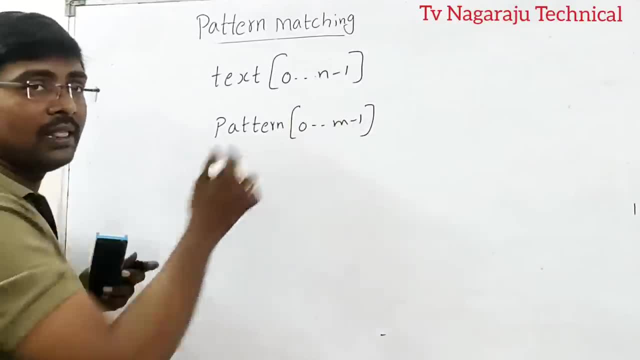 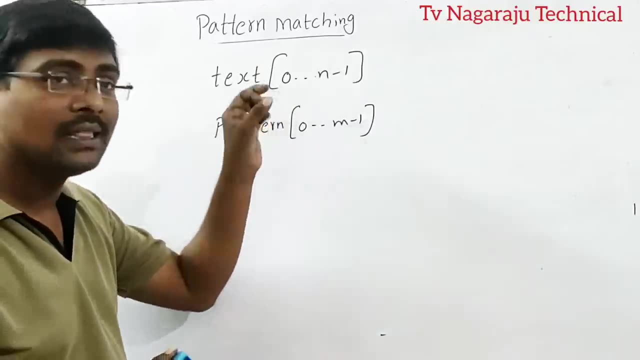 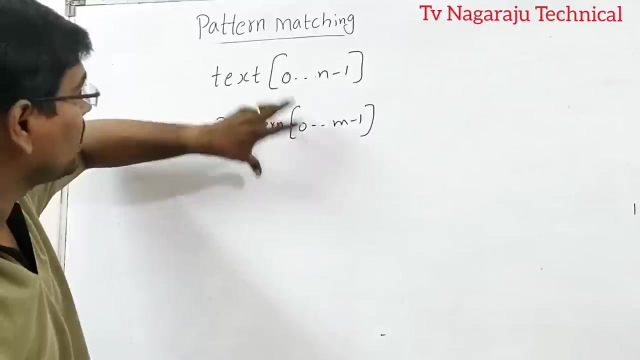 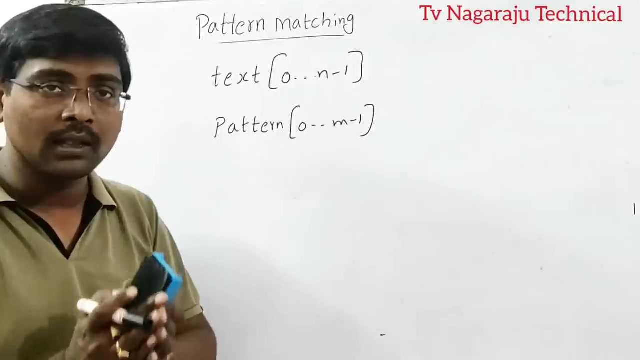 m-1.. This is also a string of length. m. Pattern matching means to check whether the pattern is available in the text or not. To test whether the pattern is available in the text or not For checking purpose, we are using different algorithms. Among them, the basic new algorithm is Brute force. 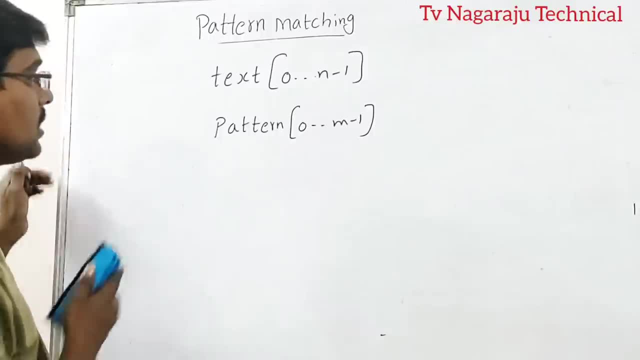 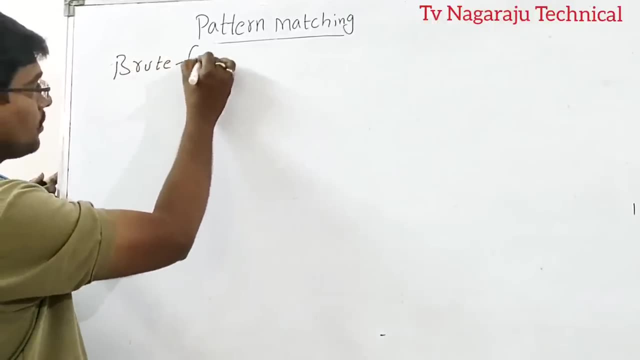 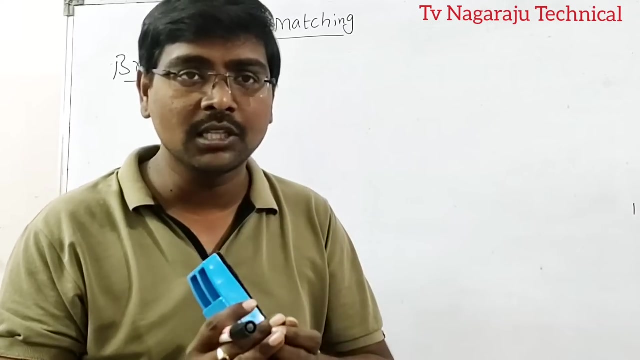 approach. Now in this session we are discussing brute force approach. Okay, Now write down brute force approach for pattern matching. First I will explain the concept. The concept is very simple. Consider two strings: One is text, Another one is line. Consider two strings: One is text, Another one is line. Consider two strings. 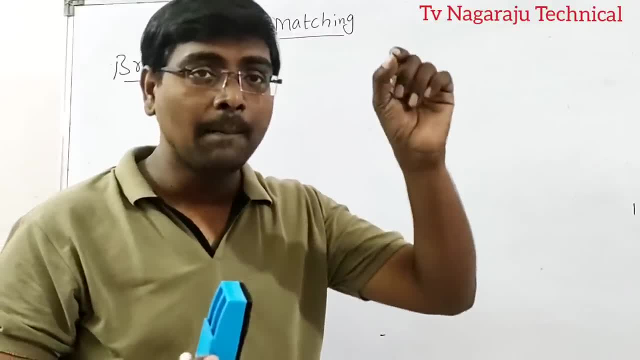 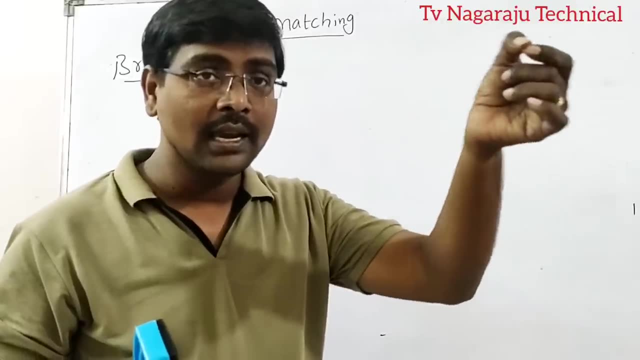 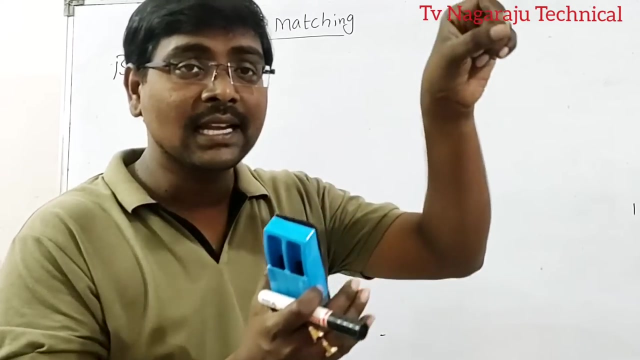 One is text, Another one is line. Consider two strings. Consider one is line, Consider pattern. the procedure is compare character by character. that means the first two character of the text is compared with the first two character of the pattern. if both are equal, move to the second character of the text. 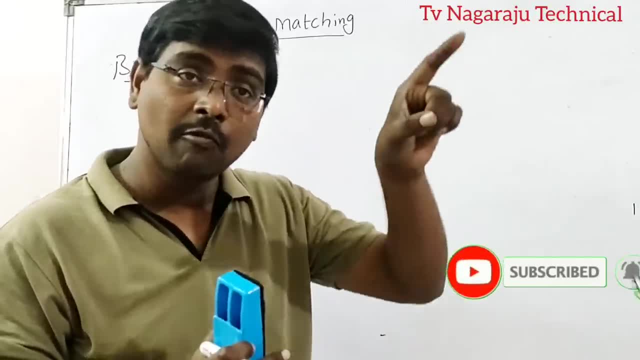 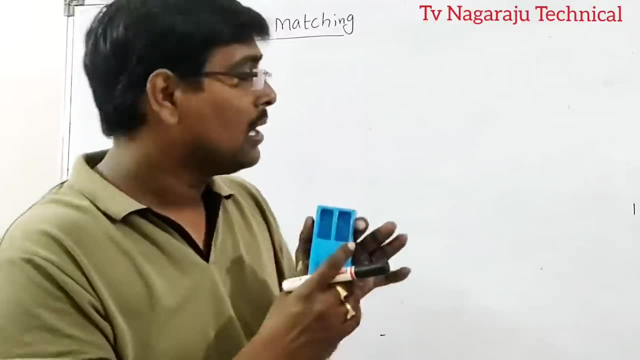 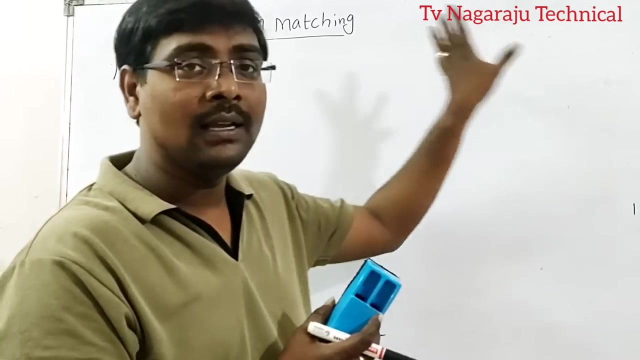 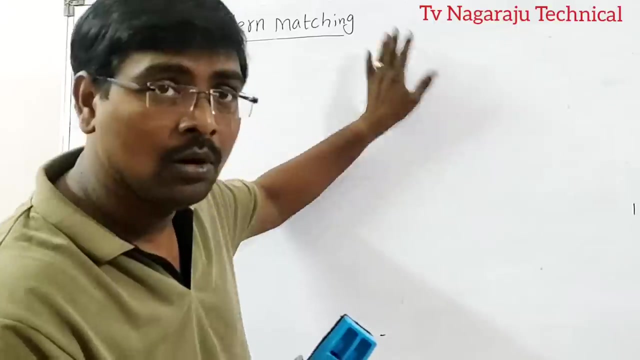 compared with the second character of the pattern. if both are matched, move to third. so the process completed until until if the complete pattern is available or if the pattern is not available, only two situations to situations is: whenever a pattern is available, no need to check the remaining. 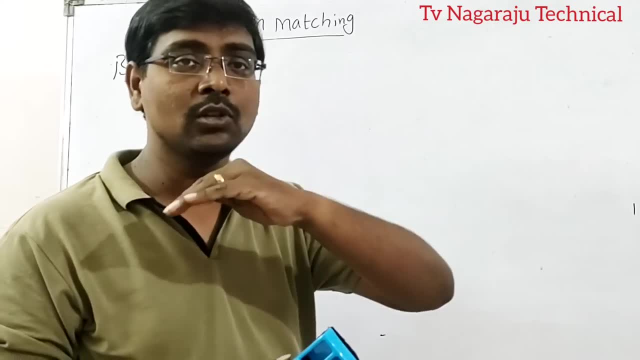 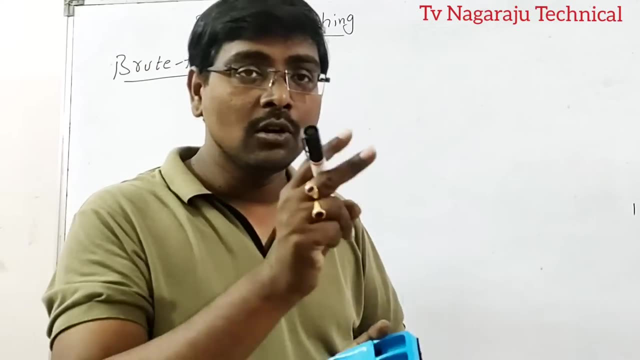 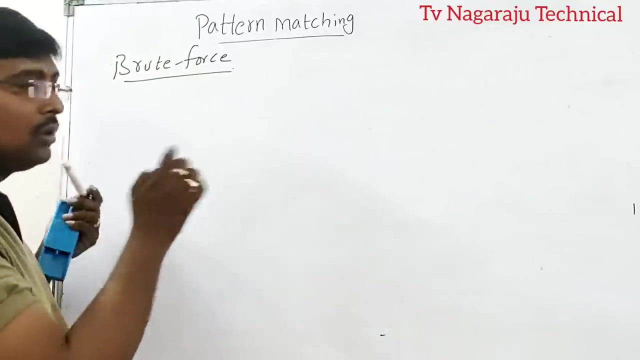 part of the text whenever the patent is available. stop the iteration or check the until text if the 를 pattern is not available. So, based on this one, we are doing the operation Now. anyway, first I will explain with one example, then you will get the clear idea. So the example. 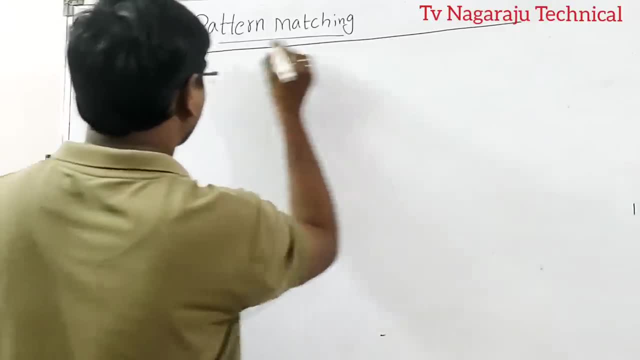 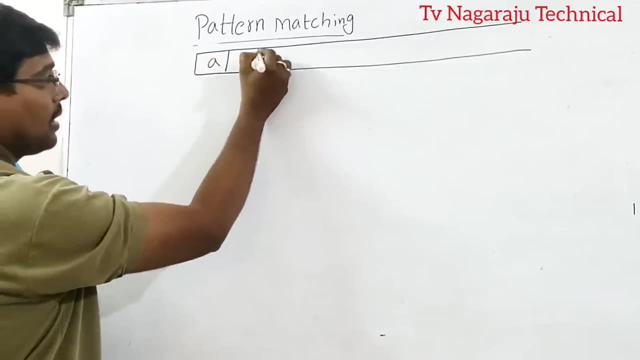 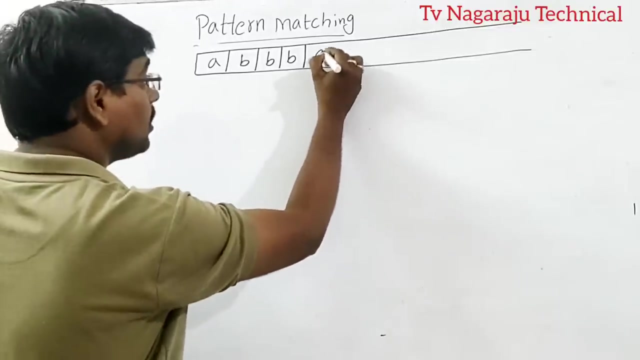 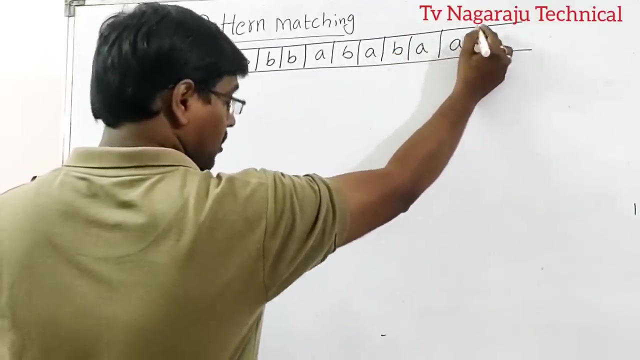 is: consider a text. After completion of the example, I will write down the algorithm: A, B B. You can take any string: A, B, B, A, B, A, B, A, A B. Suppose this is my 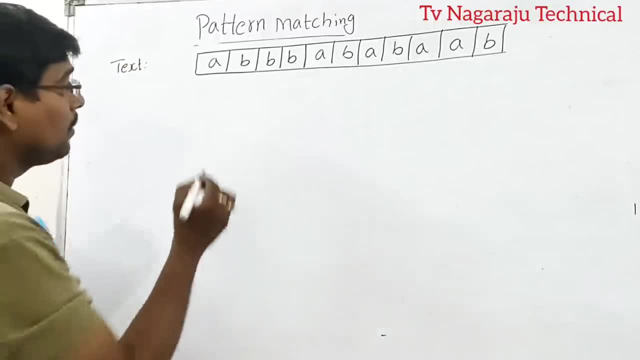 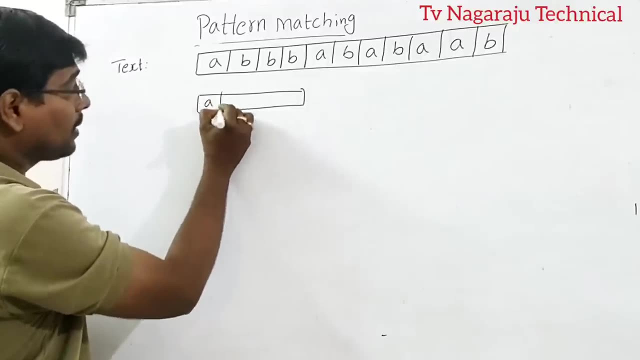 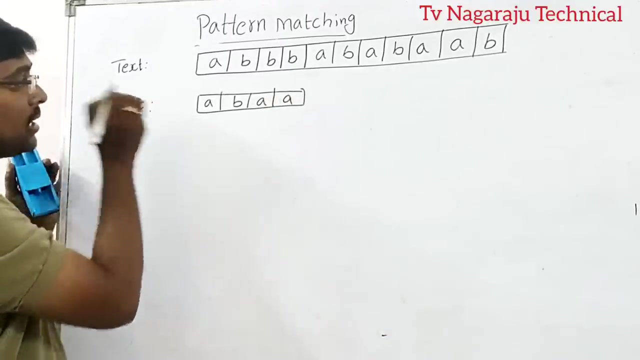 text. This is my text. Observe now, I am taking a pattern. I am taking a pattern. Assume my pattern is A, B, A. This is my pattern. Now understand the procedure carefully. So first the character. this is: 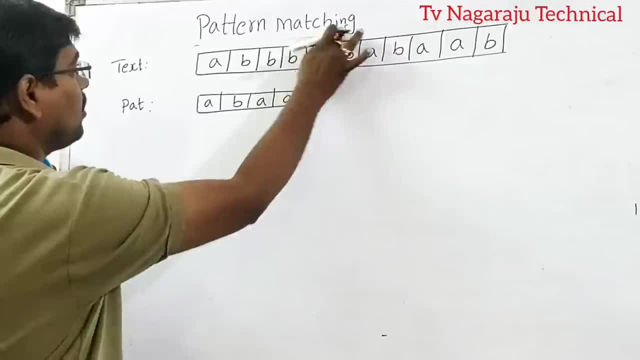 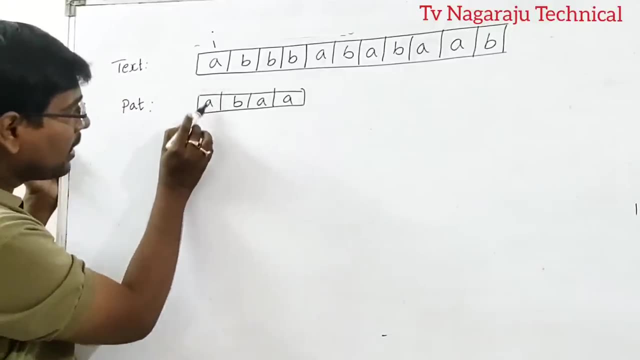 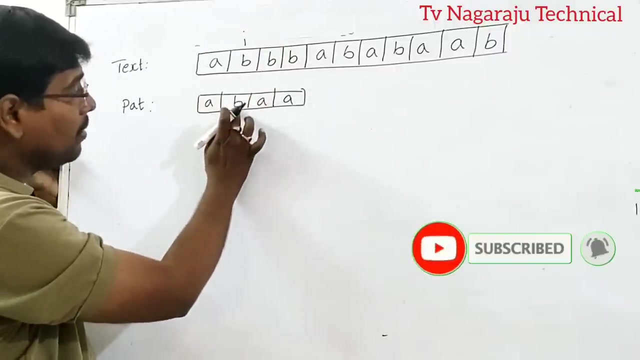 compared with this one. Assume, here I have: I am using some variable I. I am using some variable I, just for understanding A and A: both are equal. If both are equal, move to the next position. B and B: both are equal. Move to the next position. Move to the next. 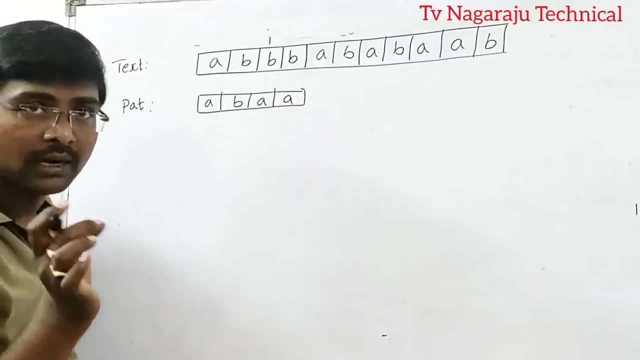 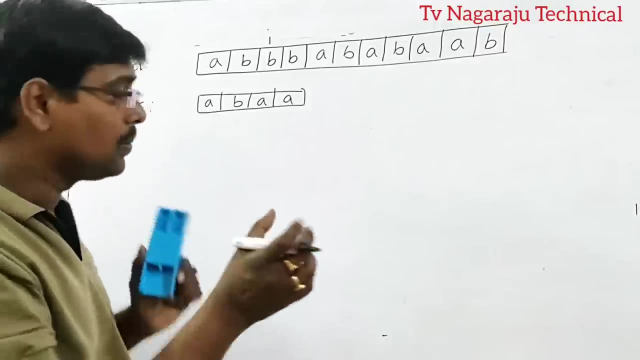 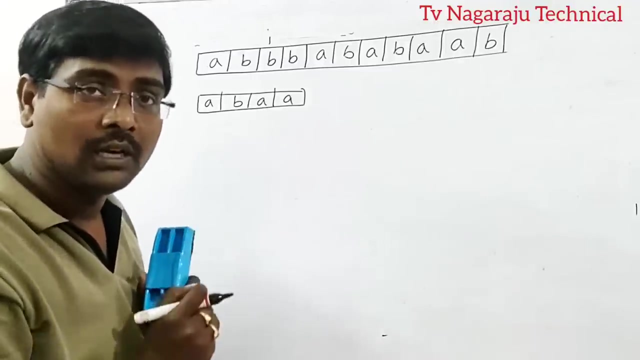 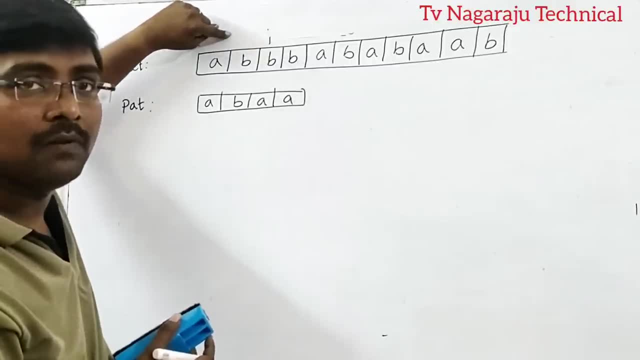 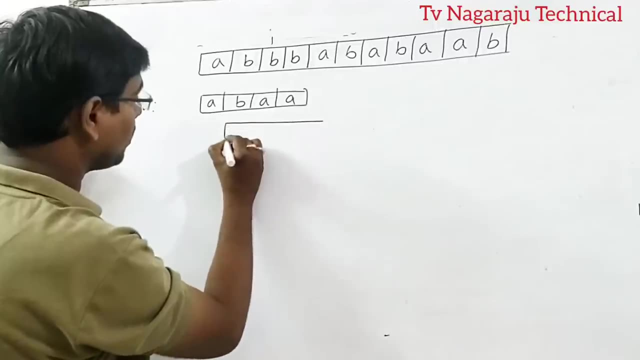 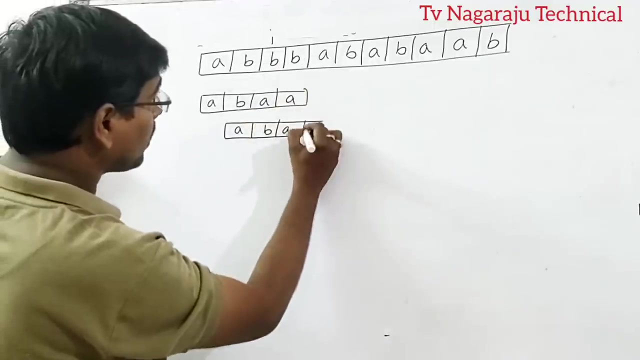 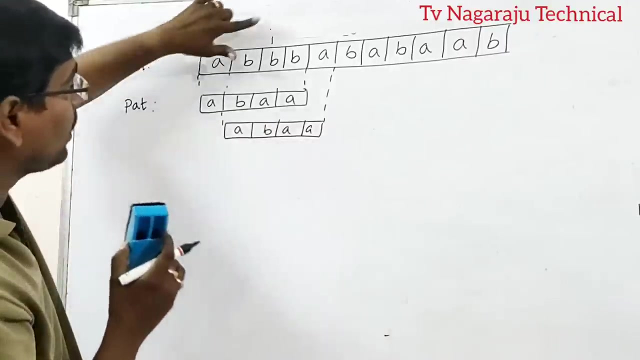 right, and again we backtrack to the previous stage. Backtracking to the previous stage. Understand So what I am doing: Shifting. Shifting means A, B, A, this one, and then A like this. Okay, Now again backtrack, Backtrack. 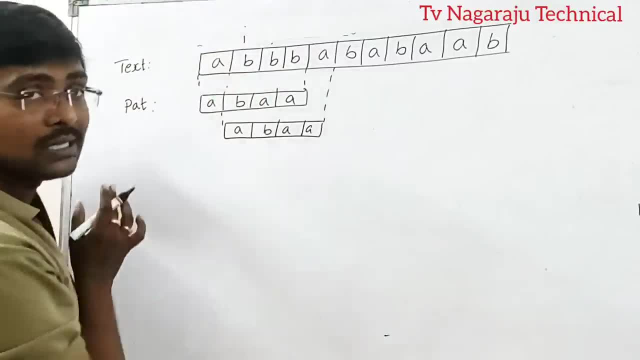 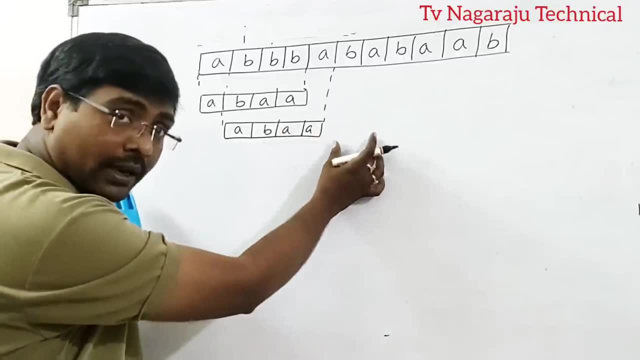 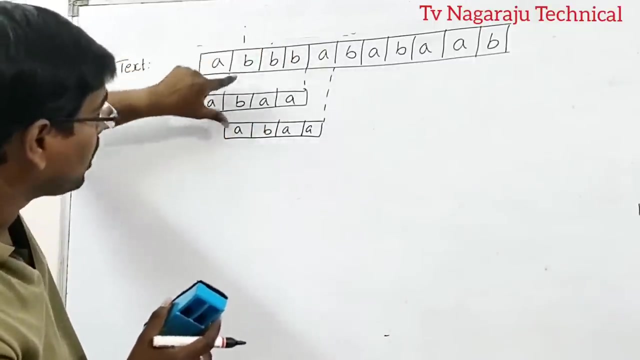 means? what is the position? This is the position Now. this is the index. So each and every time, whenever a mismatch occurred, the pattern shifted to the right side and the index again backtracked to the previous stage. Now B and A- both are not equal- Again mismatch occurred. Again mismatch occurred. 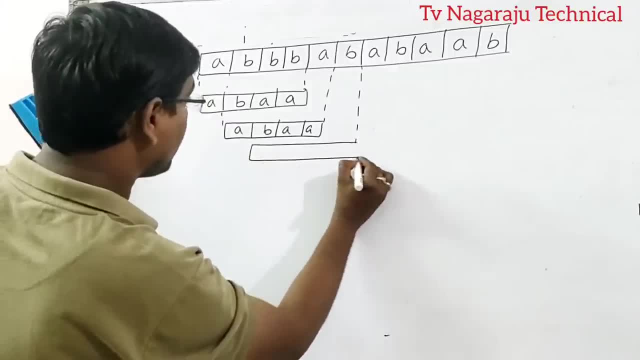 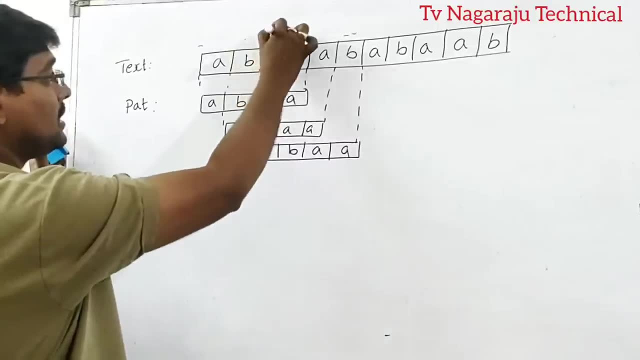 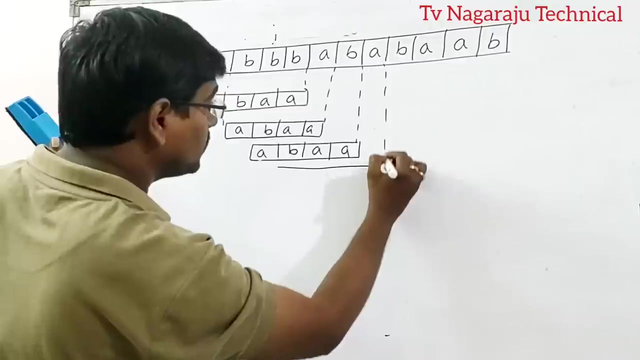 What you are doing. whenever the mismatch occurred, Again, do the same process: A, B, A, A. Now this is my index. B is compared with A. Again mismatch occurred: A B, A, A. Now this is: 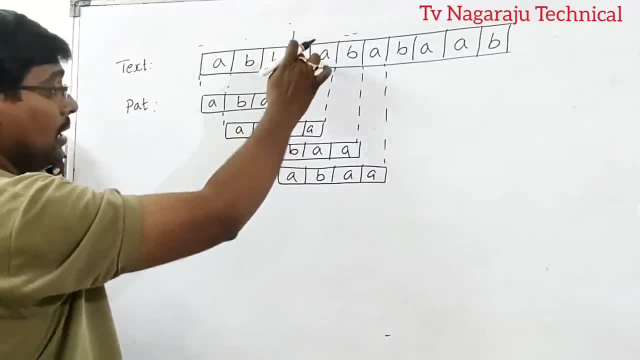 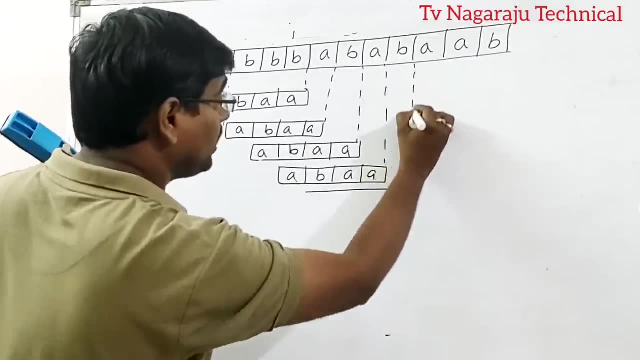 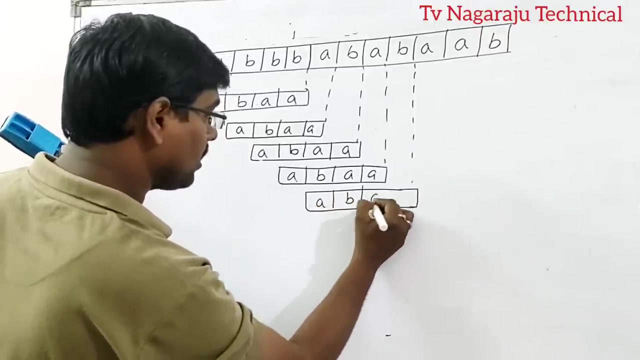 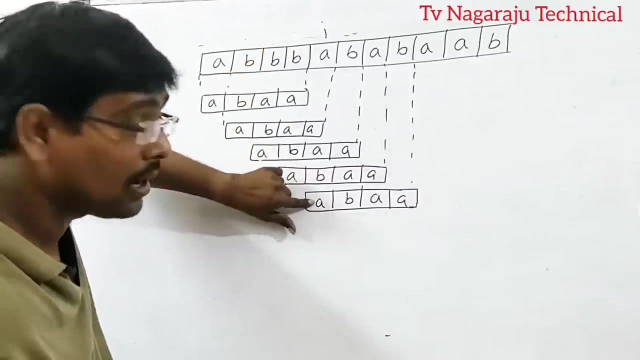 my position: B is compared with A. Again, we have mismatch. Understand, You can do, until the match Mismatch occurred, Shift the pattern to the right: A, B, A and then A. This is our position of I. Now A is compared with A. Okay, Both are equal. If both are equal, let's. 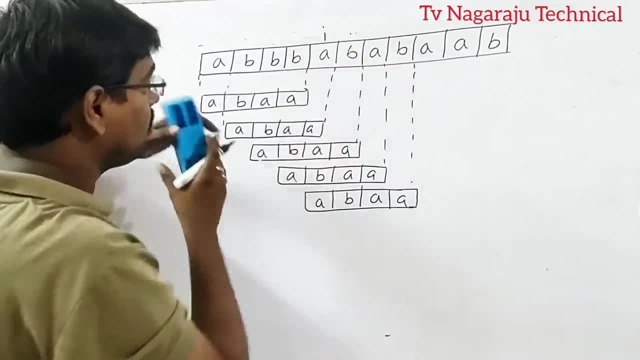 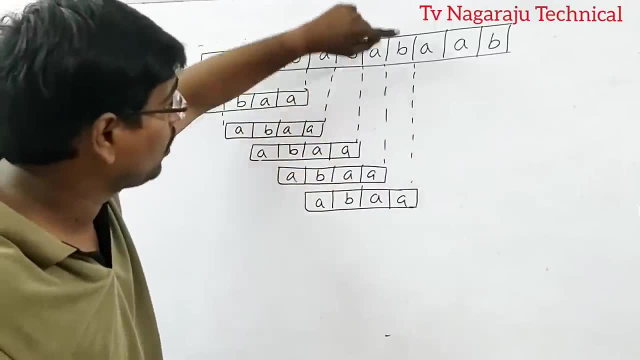 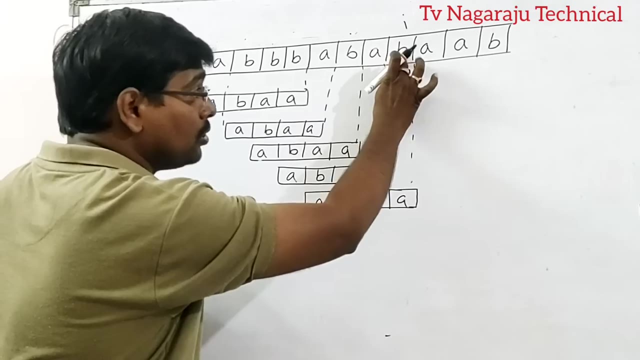 just move to this position. this is i value if both are equal next to b and b. both are equal next to a and a. both are equal next to b and a. again, we have a mismatch. actually, this is i position. at this position, b and a are. 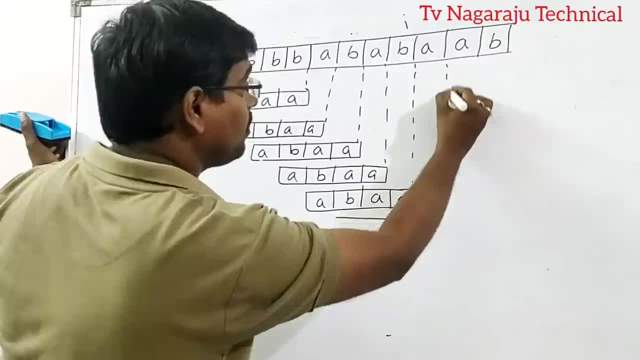 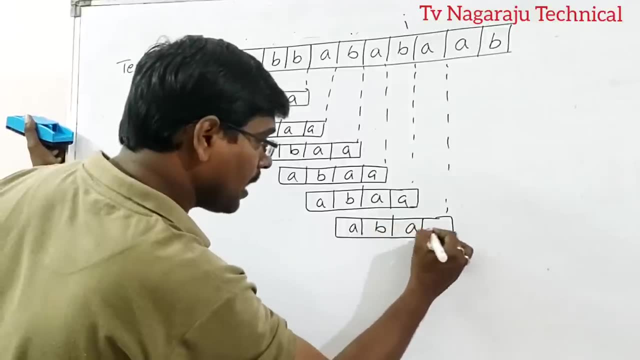 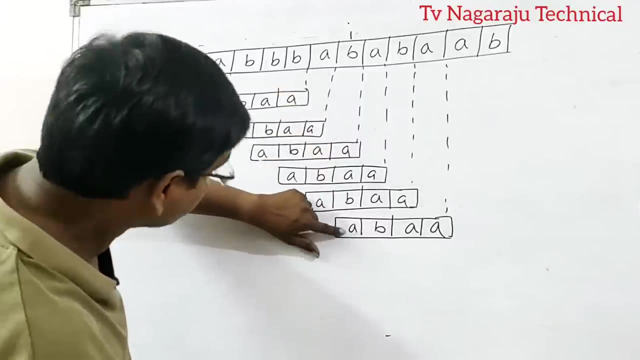 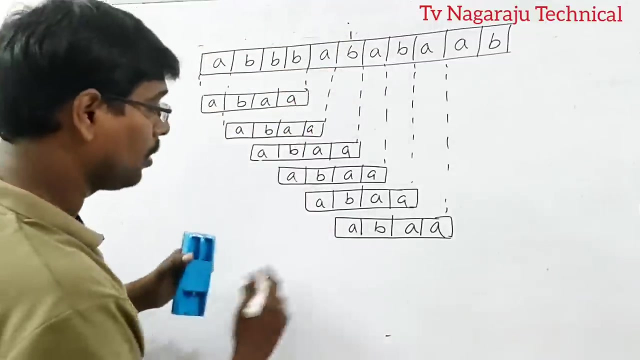 not equal. what is the procedure? if not equal means shift the pattern one side to the right. so a, b, a, a and this is the position of i. exactly very simple to remember at which position we have a in the same position i points to now. b and a matches no b and a. no matching obviously shift. 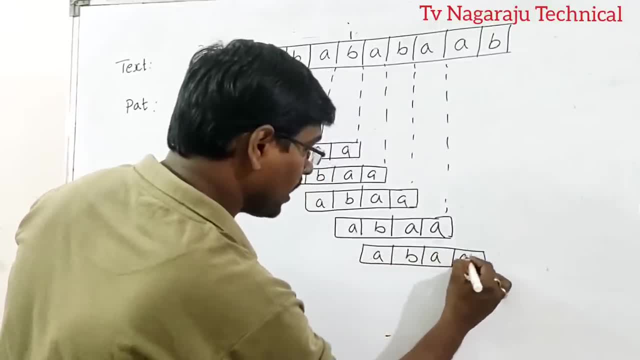 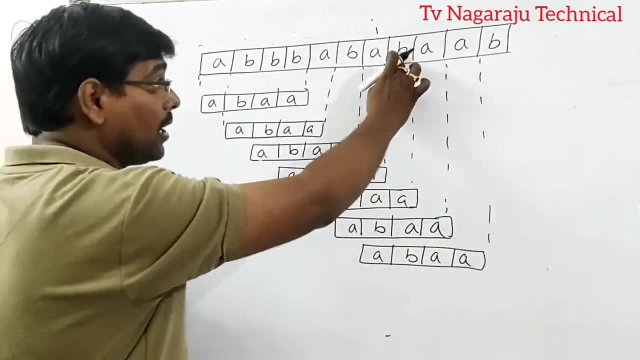 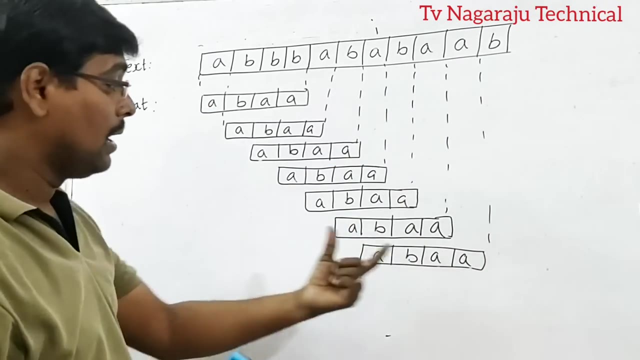 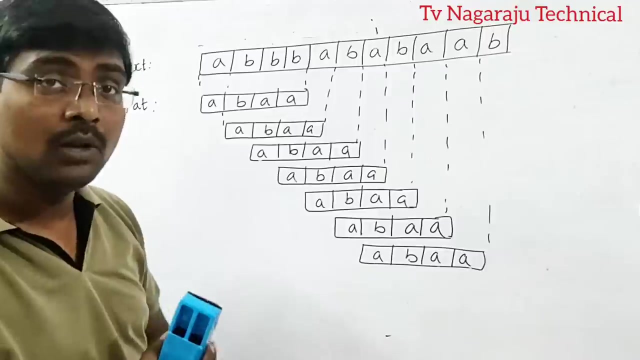 the pattern: a, b, a and a. now this is i position: a and a. both are equal. increment b and b. both are equal, a and a. both are equal again, a and a. both are equal. now my entire pattern is available in the text. my entire pattern is available in the text. 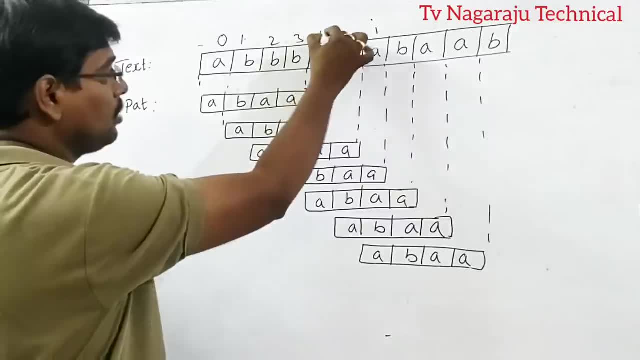 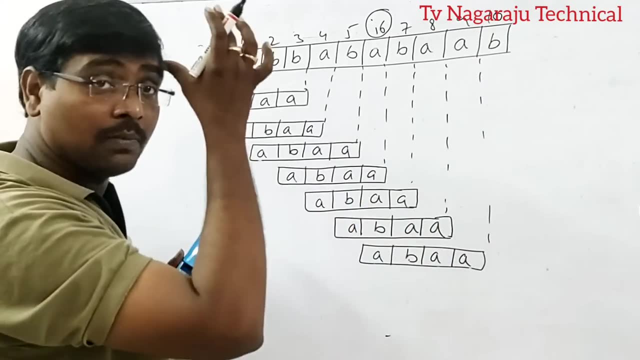 now what are the indexes? 0, 1, 2, 3, 4, 5, 6, 7, 8, 9, 10. now what is the answer? whenever the pattern is matched, it retains the index. you can see that the index is 0, 1, 2, 3, 4, 5, 6, 7, 8, 9, 10. 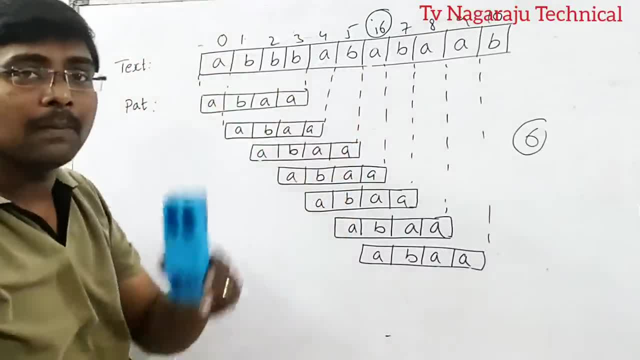 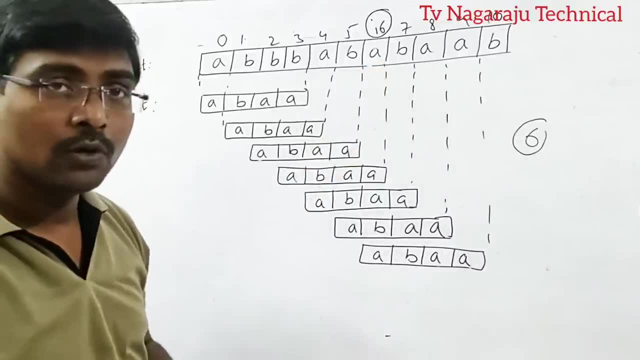 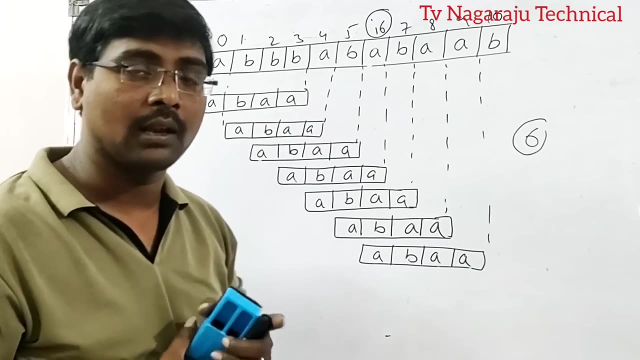 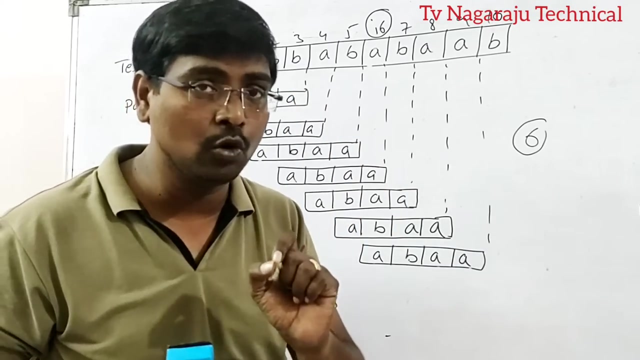 the pattern is available at index number six. this is the general brute force approach. we are following general brute force approach. we are following now for this. i will write down one algorithm. i will write down one algorithm. understand the algorithm consists of two loops. the algorithm consists of two loops. one loop is used for repetition of the text. 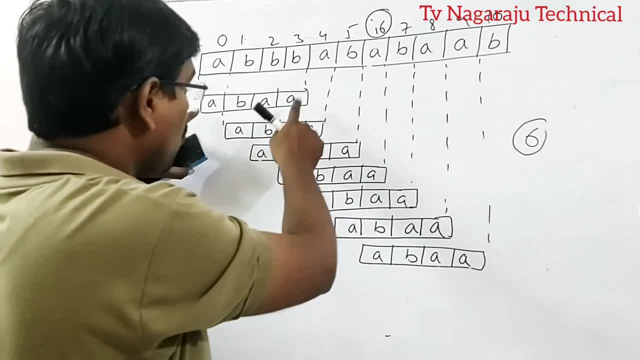 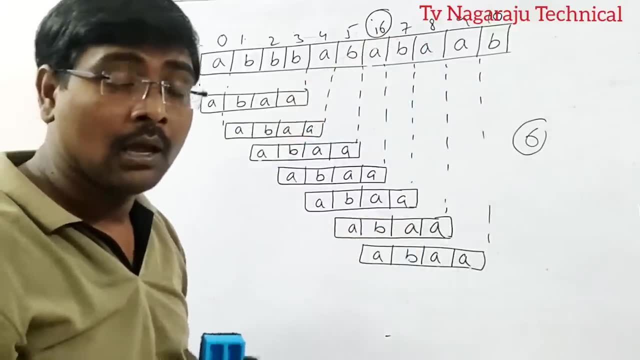 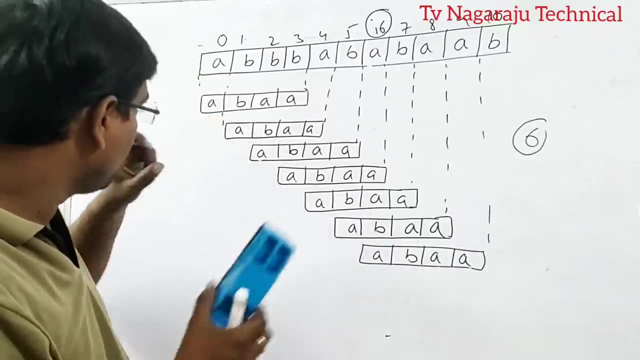 the algorithm consists of two loops. one loop is used for repetition of the text, one loop is repetition for pattern s or no one is for the text, one is for the pattern. how many number of times a pattern loop is repeated? simply length of the pattern. for example, assume a variable: j. j is equal to 0, j is equal to 1, j equal to 2, j is equal to 3. 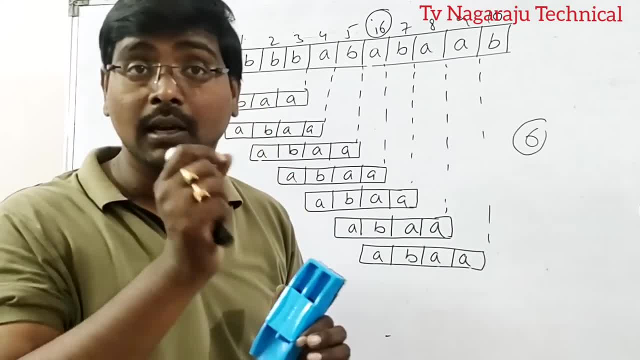 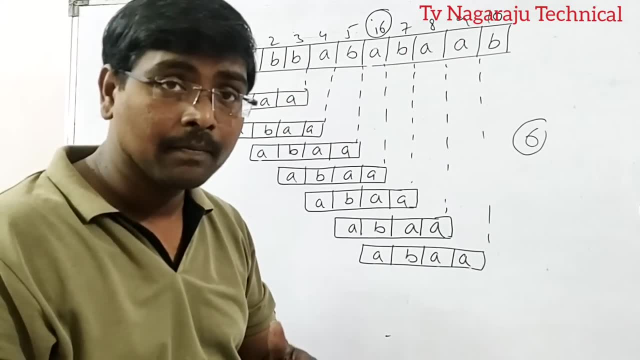 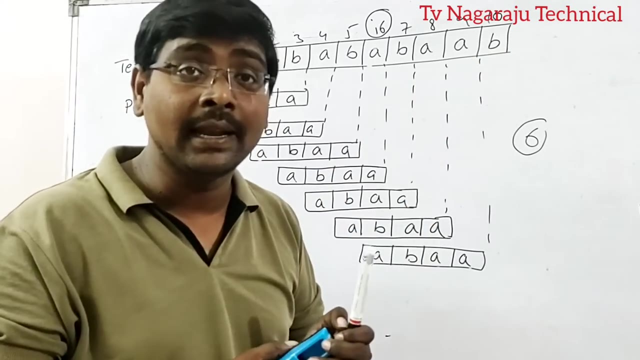 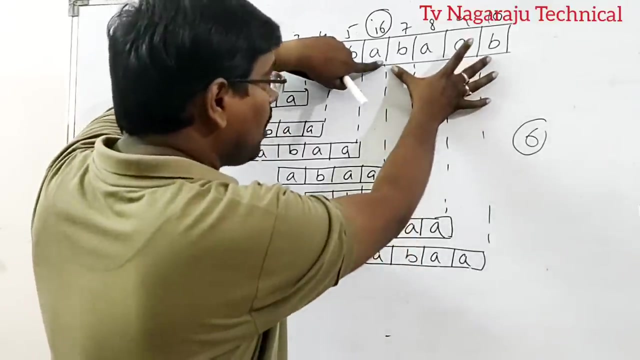 so the pattern is repeated. length of the pattern. that is good. now the important thing is how many times the text is repeated. understand carefully. so the length of the text is n, the for loop is repeated n times. no, why? because here what is the length? here four. so up to here four, whenever. 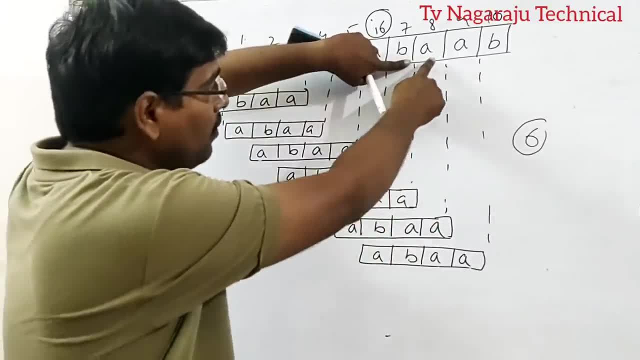 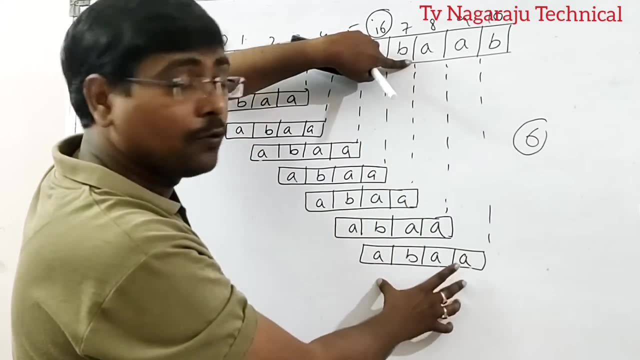 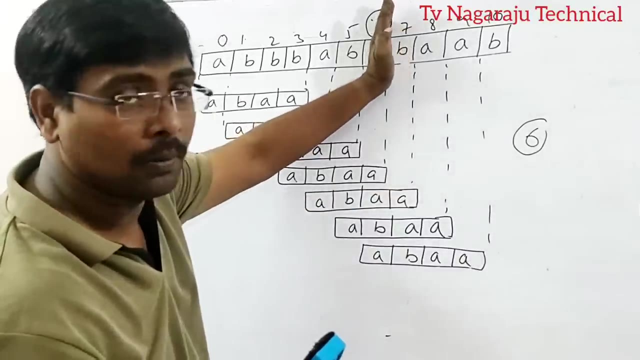 we are at the position eight. assume, whenever we are at the position eight, i have remaining three characters. yes, whenever we are at the position eight, i have remaining three characters. yes, but my pattern length is four. now what is the need of checking these three? you got my point, so up to here only no problem. and here also no problem. for example: 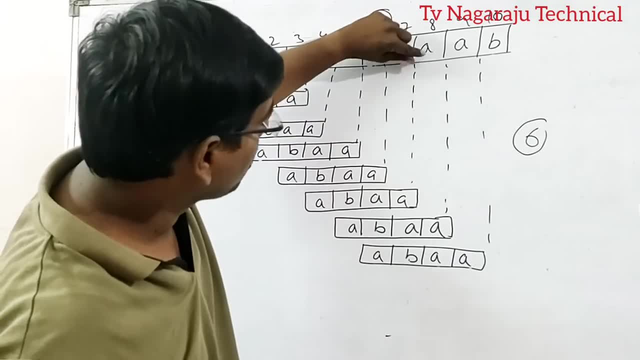 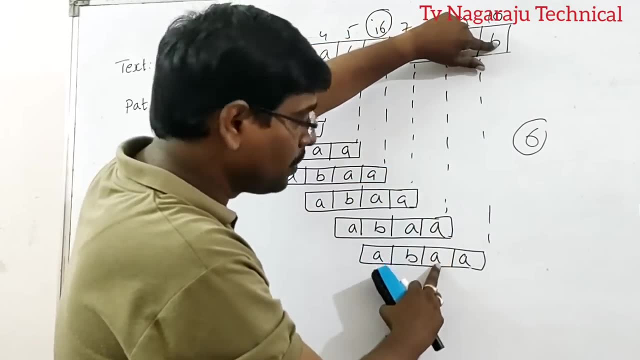 at this case also, if there is a mismatch, if you are moving this one, so okay, go to this one. a is compared with a, a is compared with a. for example, assume b is compared with b, then here there is no element, but here we have a pattern that means 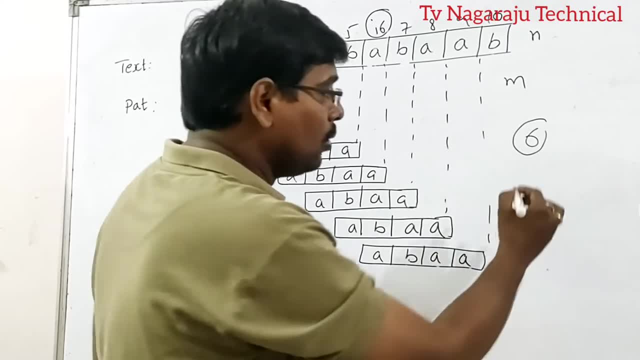 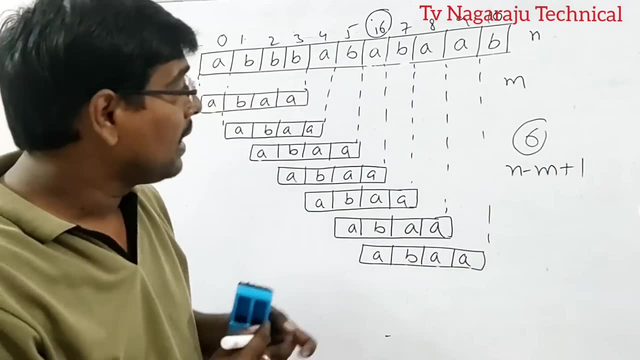 i am initial souping a and i am. next thing is i get this one. so it is not correct and, if nothing else, the problem is not right. the problem of that is you are not right. the problem of that is your position at this is the problem, so that you are constantly passing yourself. 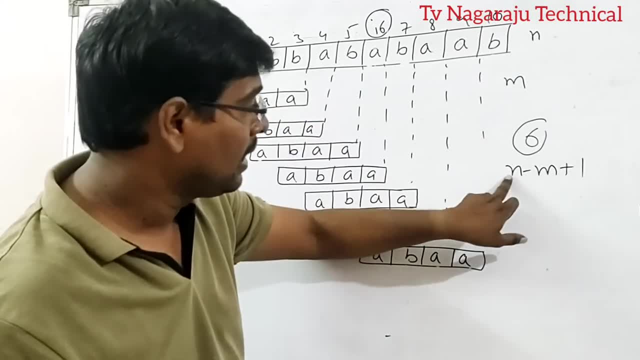 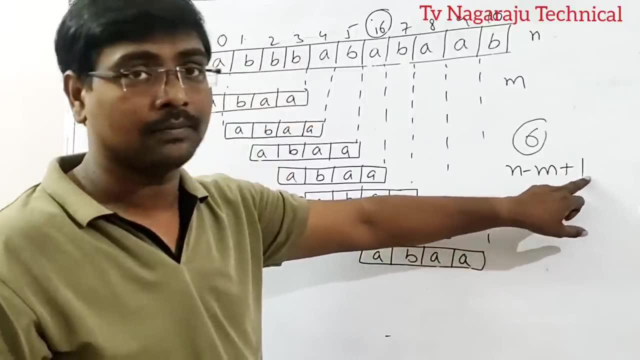 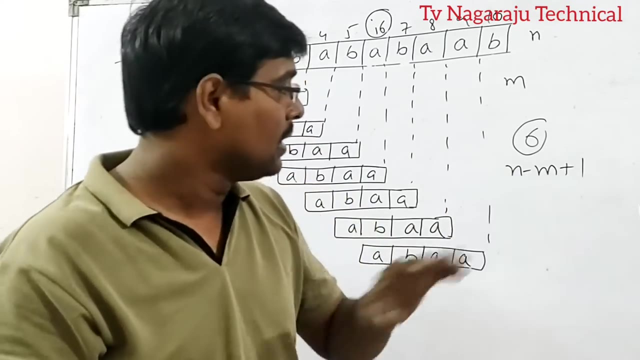 hope you all are in this game and so you will not believe it. because, um, because, if something happens, i have to change the gotcha say: wait, i didn't see this thing. wanna have a отнош to imagine if. if the sentence has the text all correct will not work. it only thing is not. 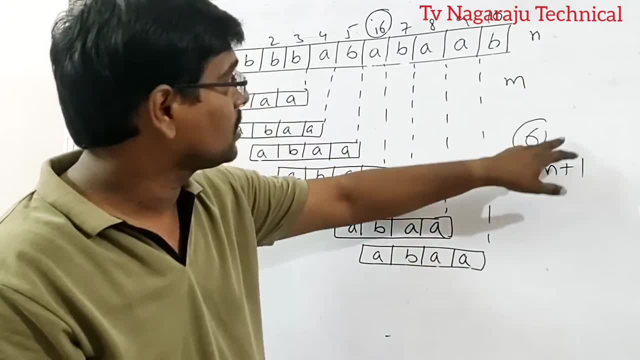 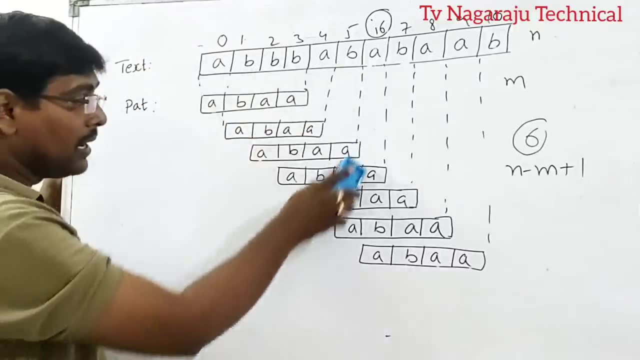 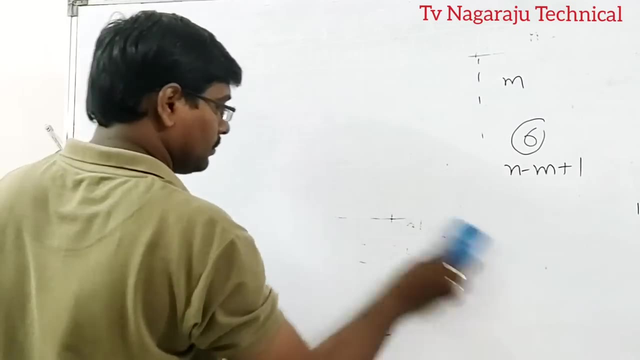 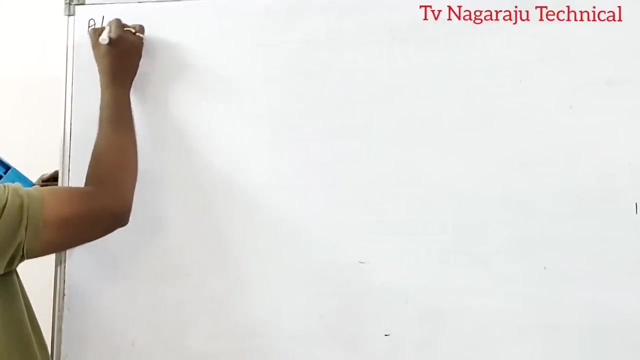 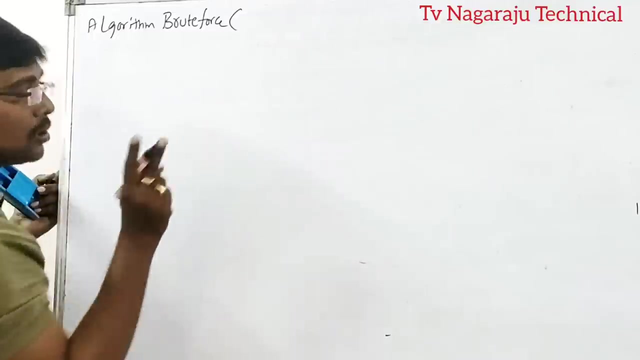 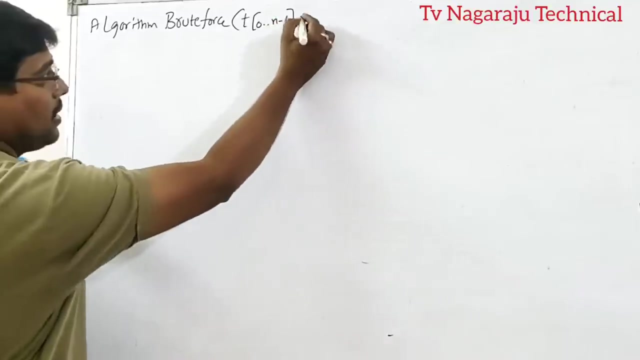 plus 1, 8. the loop is repeated only that many number of times. anyway, i will give you one example again. explain the same example by using the algorithm. first to write down the algorithm, algorithm brute force of. so take two parameters. assume the first one is t of 0 to n minus one. second one is p of 0 to m. 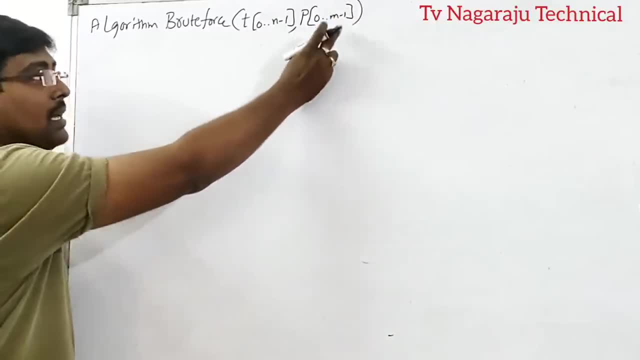 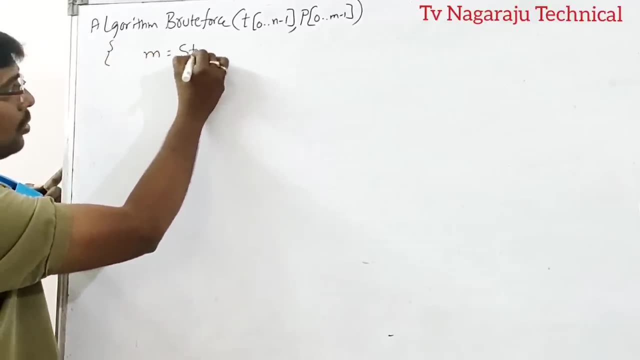 minus 1. so t is the text, p is the pattern, p is the text, p is the pattern. if you are in it out, you can write like this: suppose m is equal to htr ln of p. now what else is of? m consists of the length of 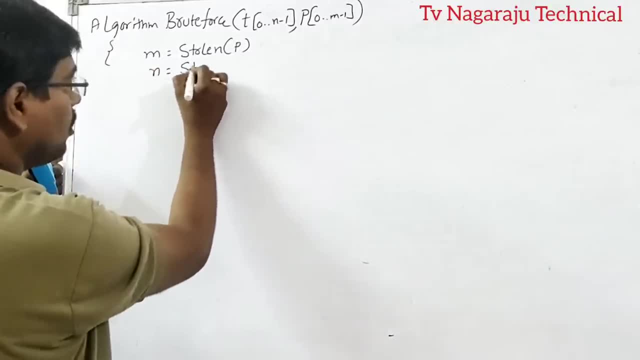 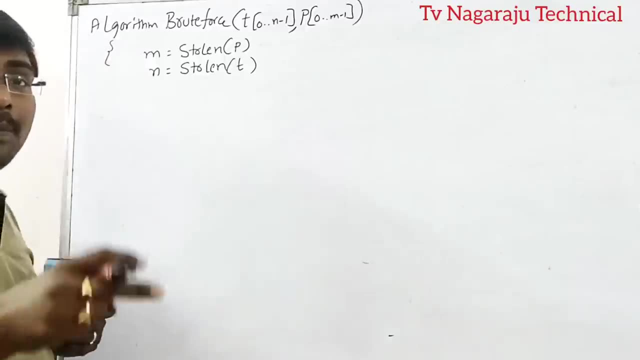 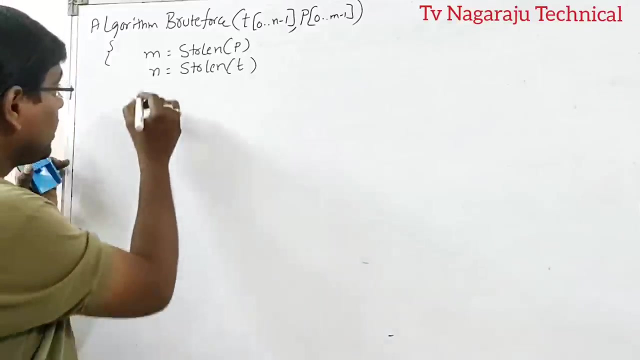 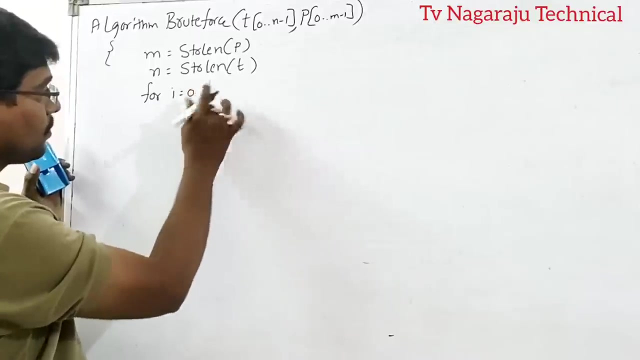 this: the pattern: n is equal to strlen of t. n consists of the length of the text. Now repeat a loop: up to n minus m- number of times, Yes or no? Up to n minus 1: number of times, For i is equal to 0, i less than or equal to n minus m, If you are writing equal to that. 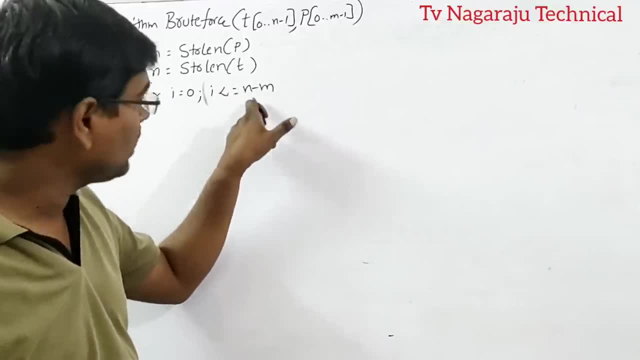 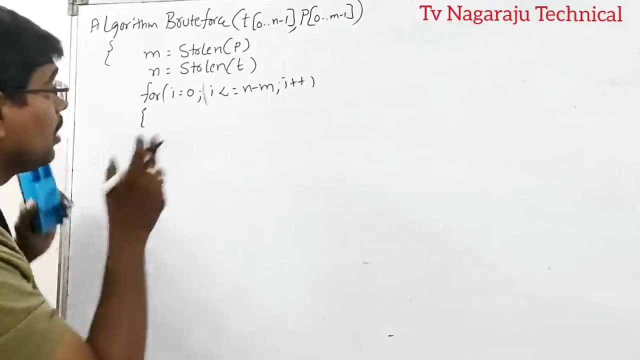 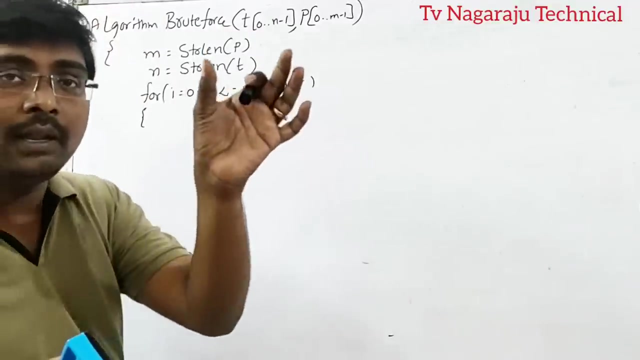 is the reason: n minus 1.. Suppose, if you are using only less than n minus m plus 1.. So i plus plus Within the loop. what we are doing? This is the loop for repetition of text. The i is the variable index for repeating text. 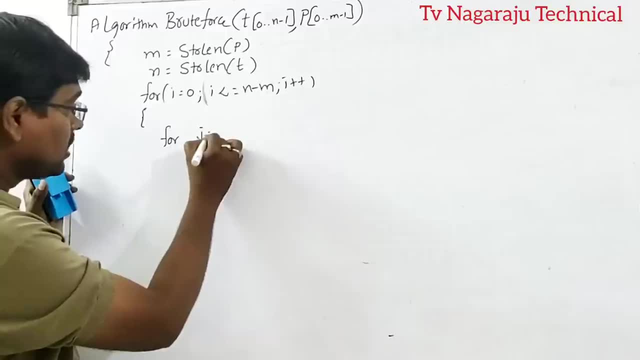 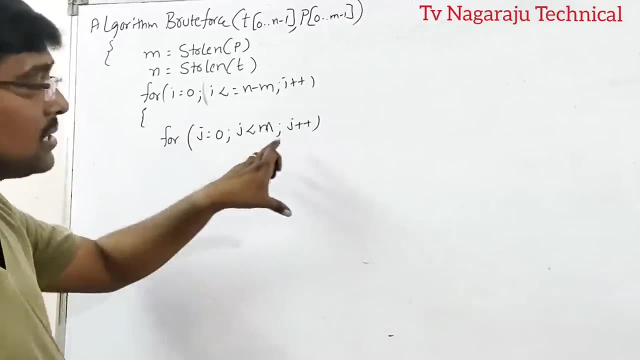 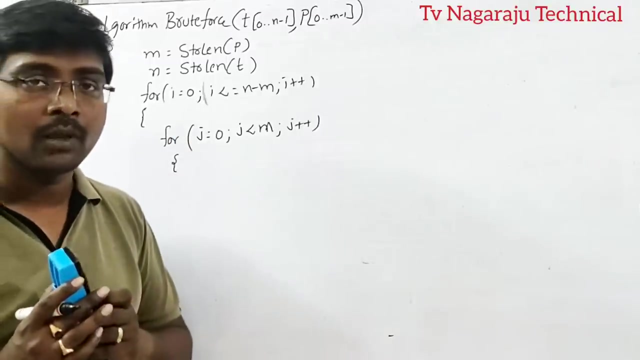 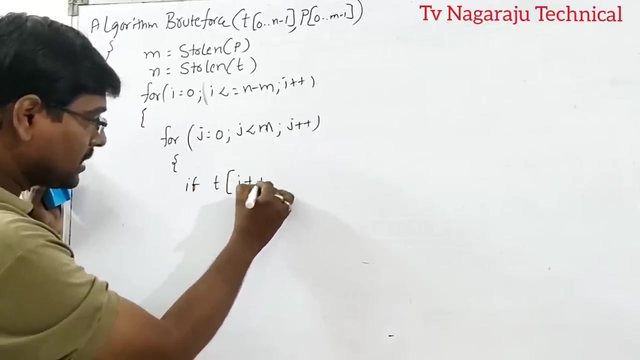 Now for j is equal to 0, j less than m, j plus plus. You got it. This is the loop for repetition of pattern. Within this one, I am writing one condition. What is the condition? Simply, if t of i plus j- Anyway, you will understand, Very, very simple- Is not equal, 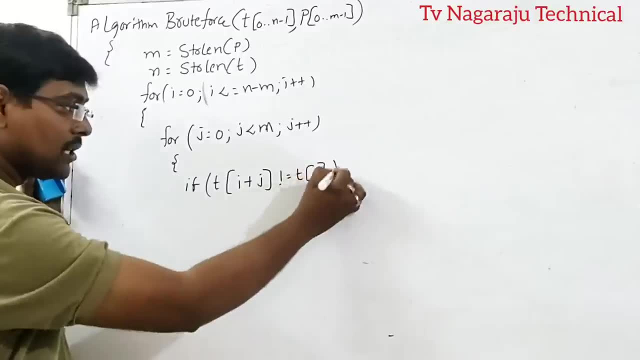 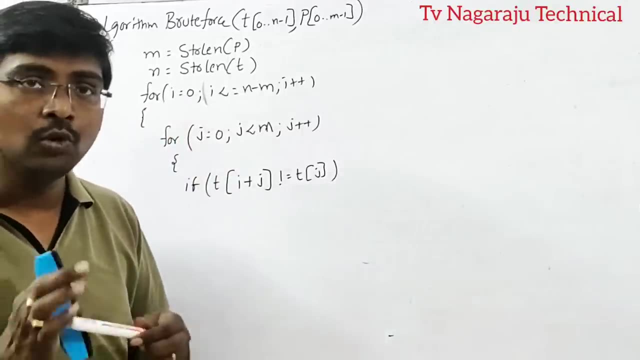 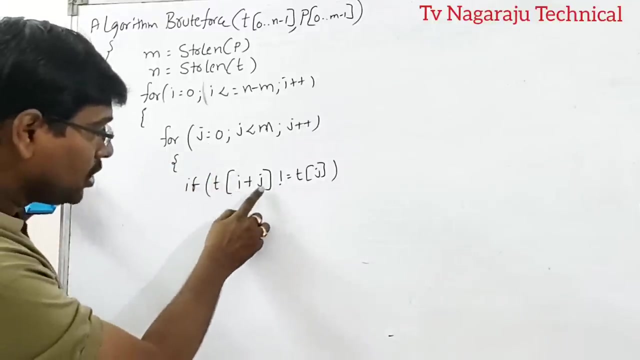 to t of. j Understand the process t of i plus j First time. i is equal to 0.. Assume i is equal to 0,. j is equal to 0.. Yes or no? Now t of 0 plus 0 is not equal to t of sorry. 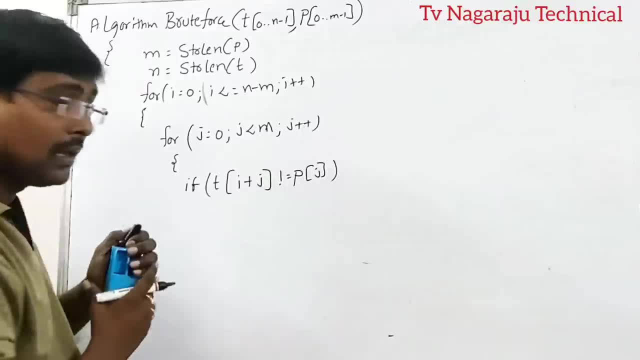 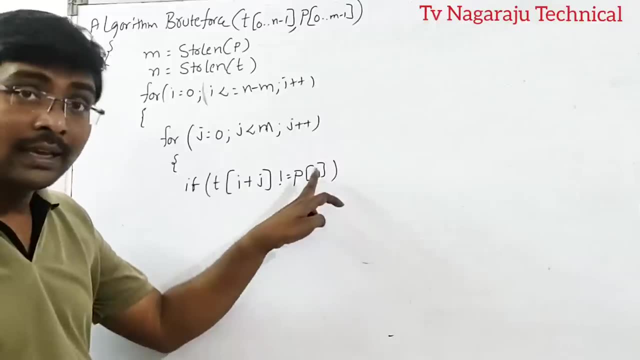 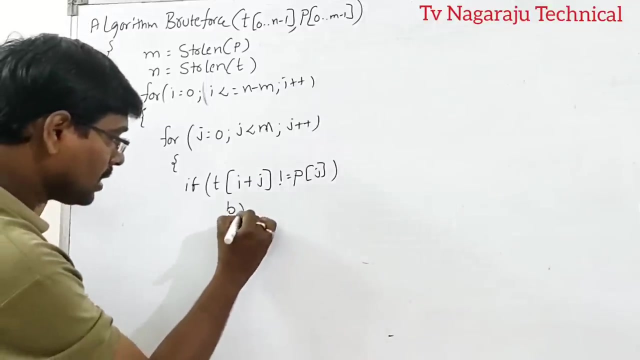 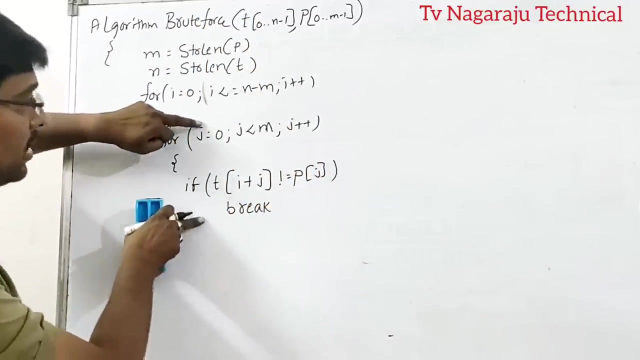 is not equal to t of j. That means the zeroth position character in the text Is not equal to zeroth position character in the pattern. So if that is the case, you are simply using break. If the first character is not matched means no need to repeat this. 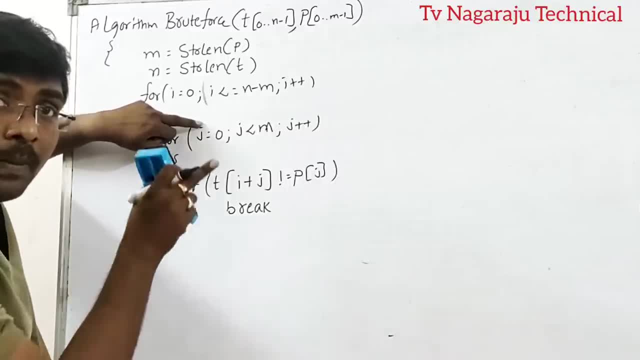 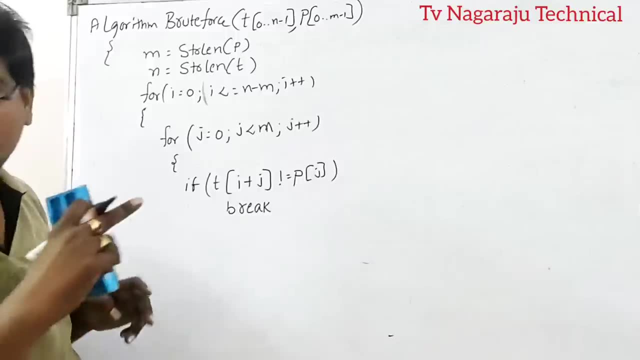 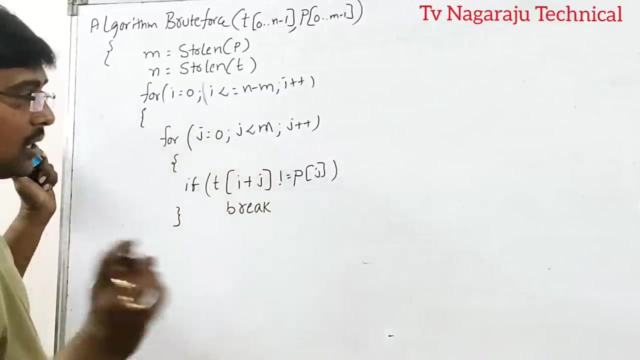 loop, Yes or no? If the first character of the pattern is not matched with the text, then no need to repeat the loop for remaining characters. Repeat the loop for remaining characters Whenever there is a match. we are doing the operation. Anyway, I will explain. 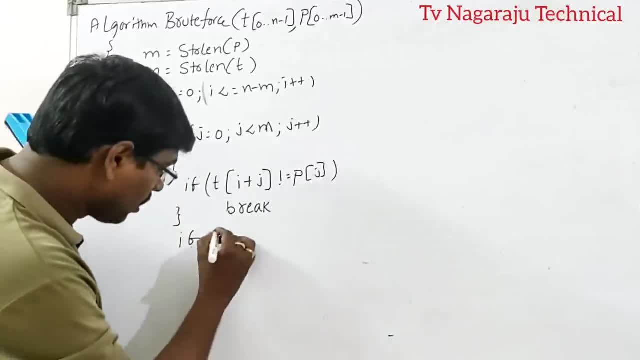 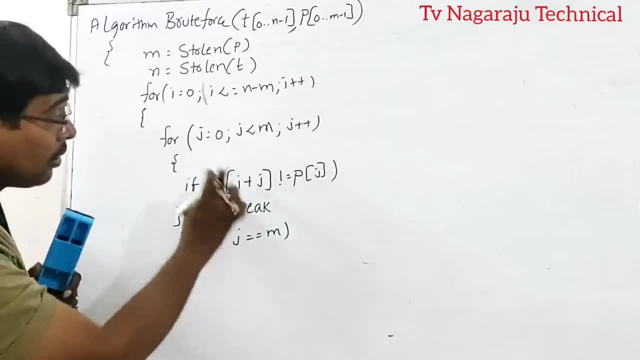 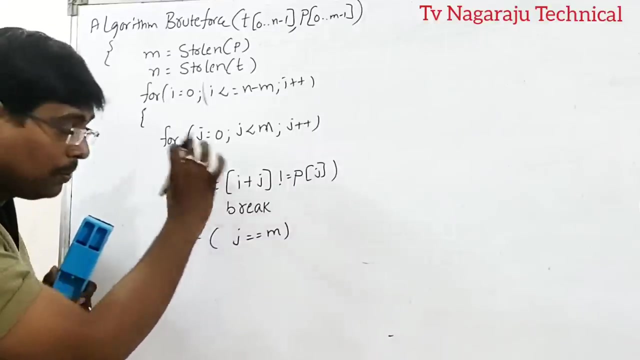 After coming out of the loop. after coming out of the loop, if my j value is equal to equal to m, So we are repeating the loop up to m minus 1.. Suppose, by the completion of the loop, if j is equal to m means the complete pattern is completed. 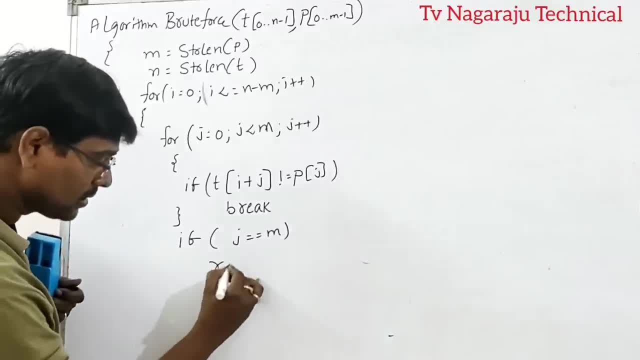 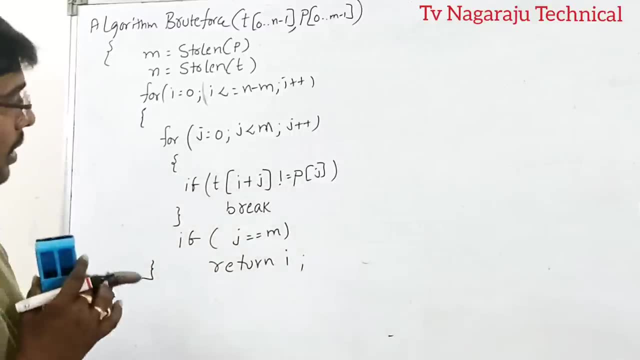 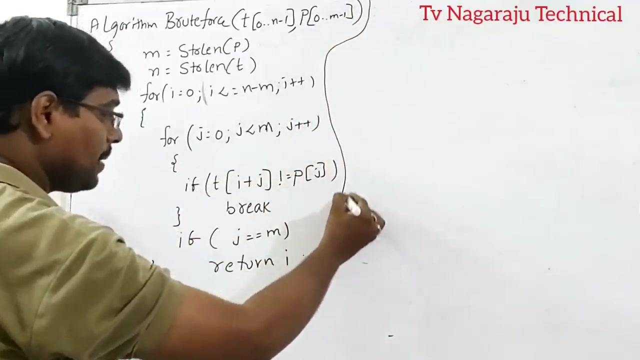 Starting with this index. So what is the answer? The answer is written. i Close the for loop, Close this algorithm. This is the brute force approach for pattern matching. Anyway, I will explain the same example. I will explain the same example by using this: 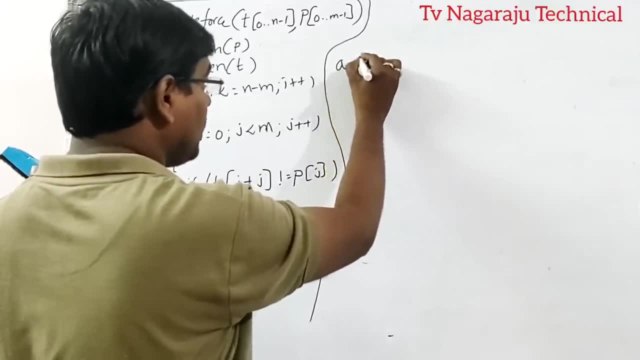 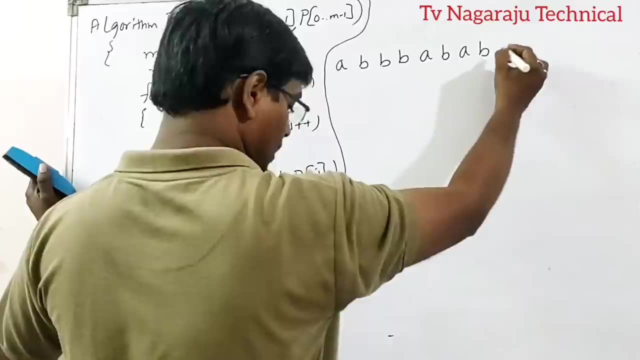 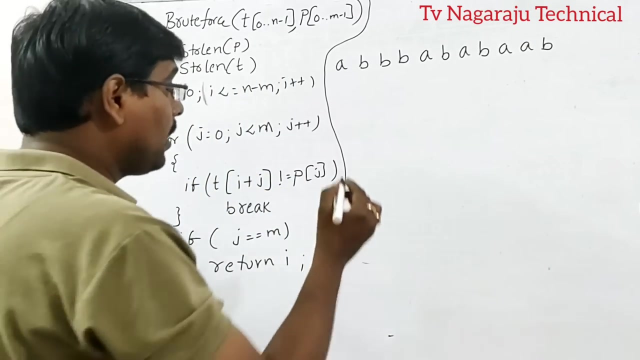 algorithm. So what is the example? a, b, b, d a, b a, b, a a b. So this is my text And what is my pattern? a, b a a. This is: 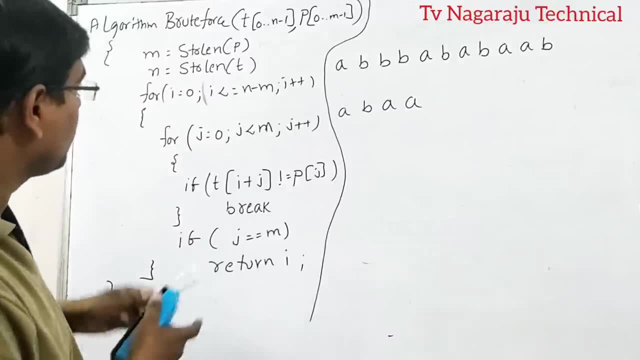 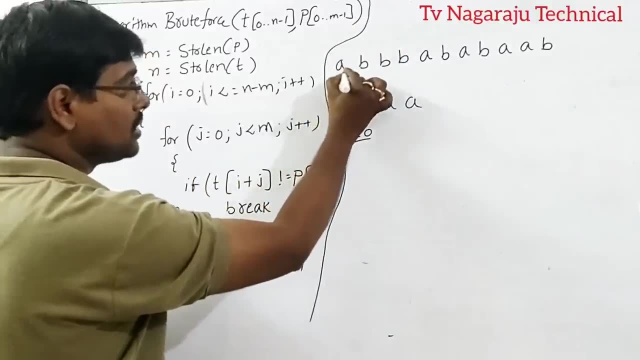 my pattern, Yes or no. Now observe the algorithm and follow step by step. In the initial stage, i is equal to 0.. So this is the 0th position: 0, 1,, 2,, 3,, 4,, 5,, 6,, 7,, 8,, 9,, 10,, 11,, 12,, 13,. 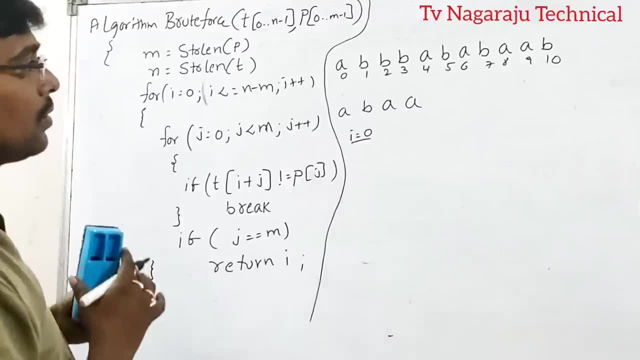 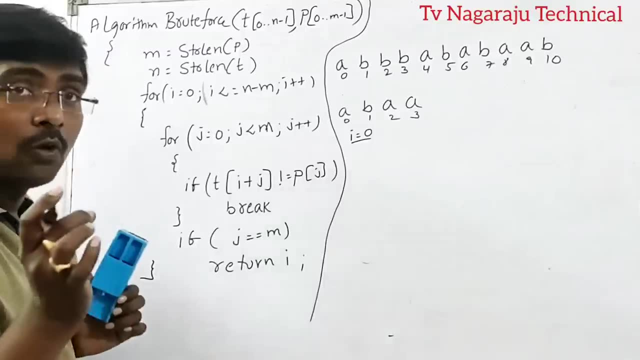 14,, 15,, 16.. Whatever it is, whatever we are getting, not a problem. So previously I have written some additional 1.. 0,, 1,, 2,, 3.. Now, first time, i is equal to 0. And 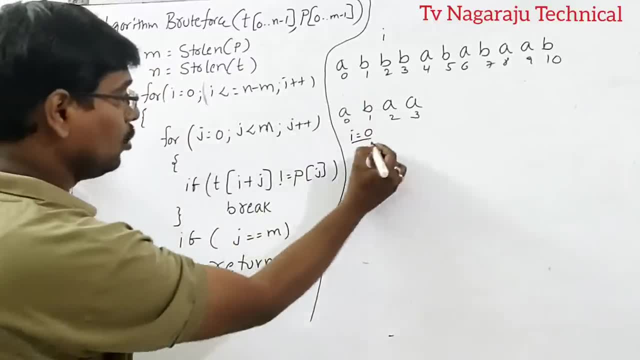 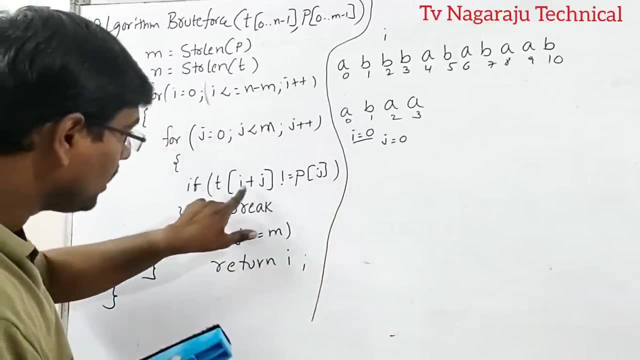 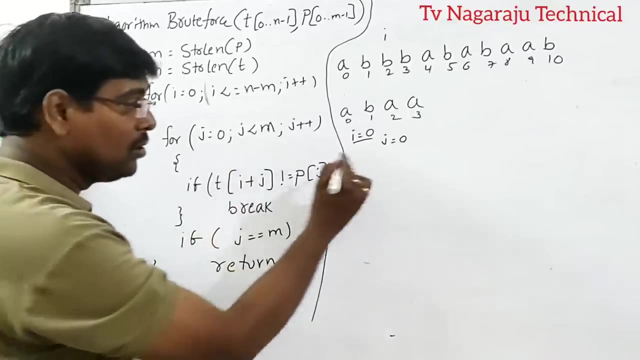 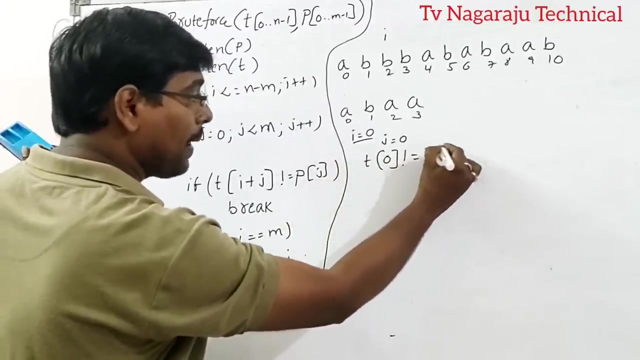 this is- i Enter inside the loop Here: j value is equal to 0.. j value is equal 0.. Compare t of Why I have written i plus j, You will understand. i value 0, j value 0.. So t of 0 plus 0 is not equal to pattern of 0.. Yes or no Check. 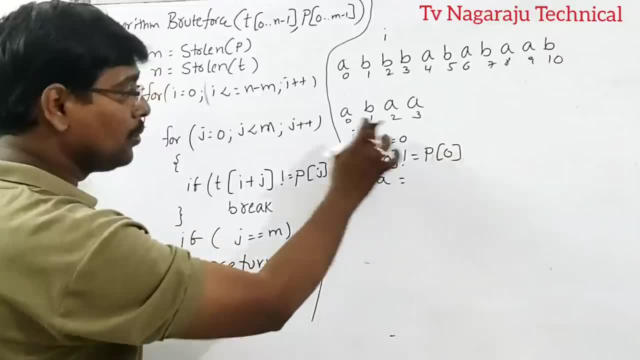 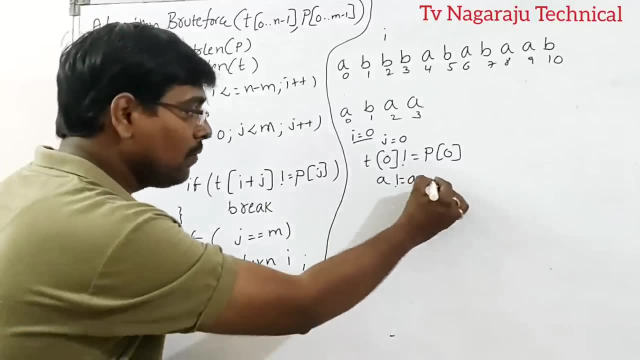 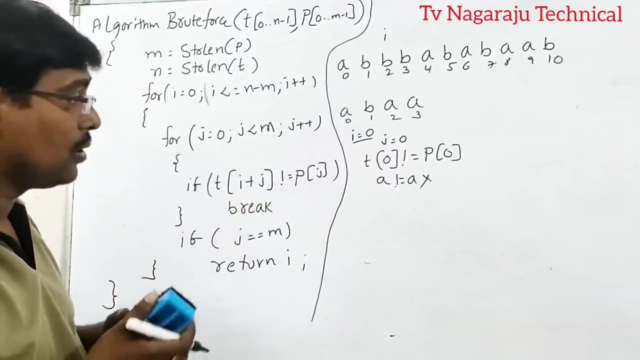 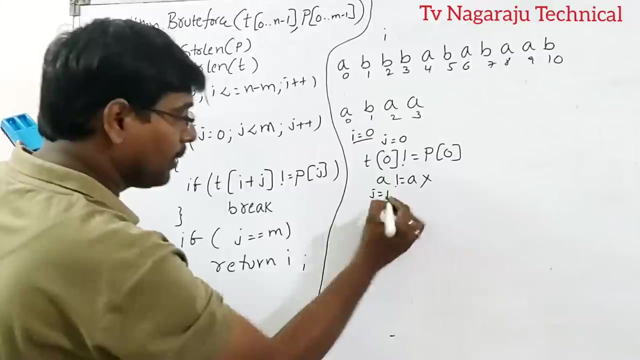 Here the value is a. Here: 0 position. The value is a. a not equal to a Condition. true or false, Condition false, Yes or no. Actually, a equal to a Condition false If the condition false means break is not executed. Now what happened? Break is not executed Now j is equal to 1.. 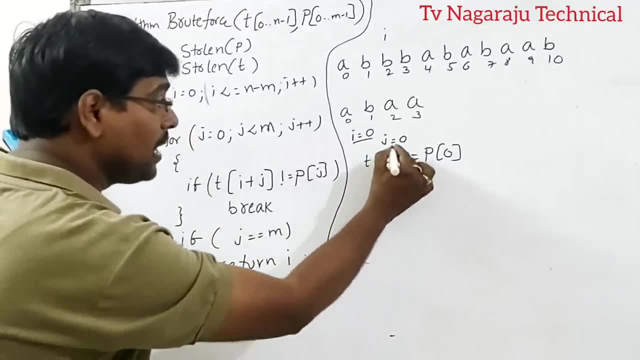 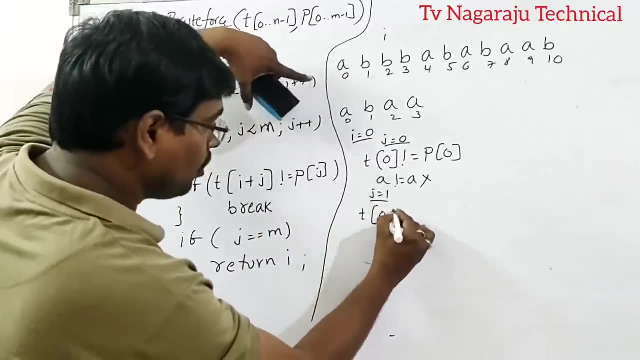 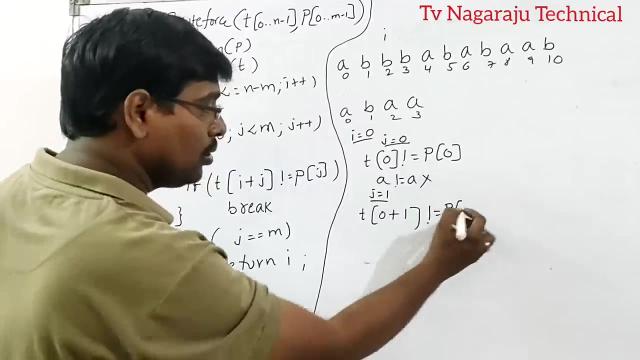 Inside the for loop. We are inside the for loop. j is equal to 1.. Understand why I written this one: t of 0 plus 1.. i plus j, 0 plus 1 is not equal to t of 1.. 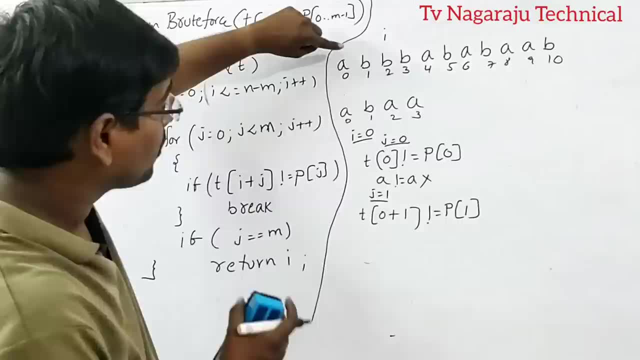 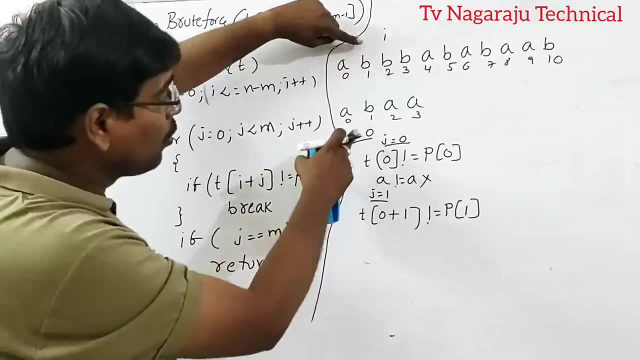 Now you got my point. Why I written i plus j First. I am making i is equal to 0. Now j is equal to 0. If both are matched, Now what is the position of this one? i plus j. So j is equal to 1.. If j is equal to 2,. 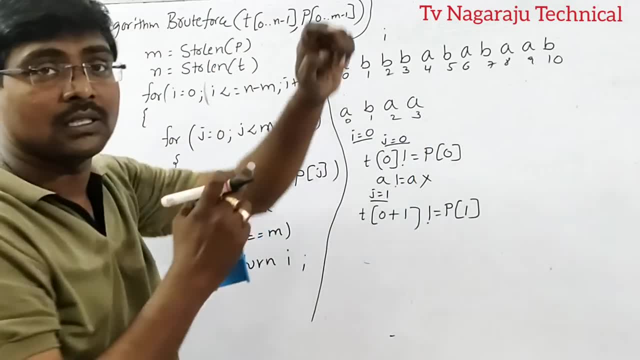 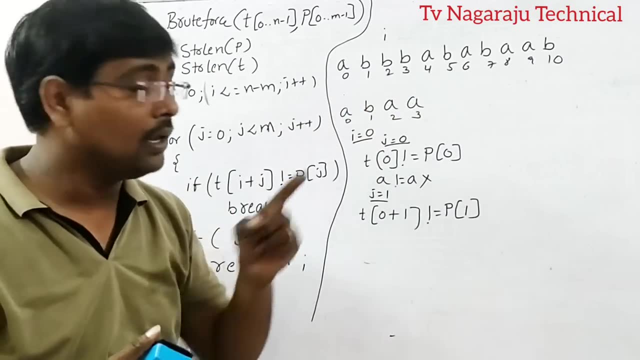 this is i plus 2.. j is equal to 3, this is i plus 3.. So whenever j value moved, I am moving this position, But you do not need to update i value Why? Again, if there is a mismatch, we backtrack. 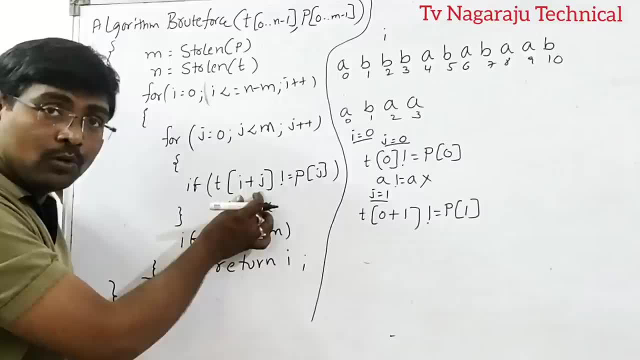 to the previous position. So j is equal to 1.. j is equal to 1.. j is equal to 1.. j is equal to 2.. previous one. That is the reason I am not using incrementing. i value So t1.. What is the value? 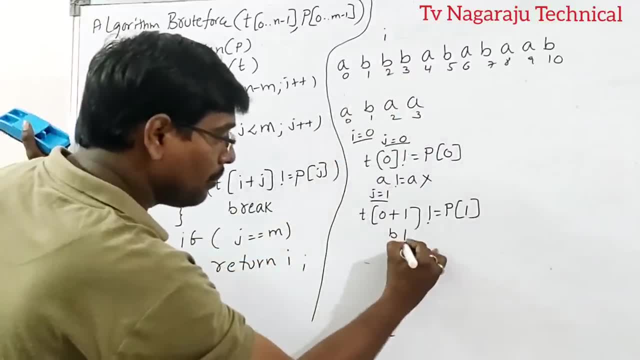 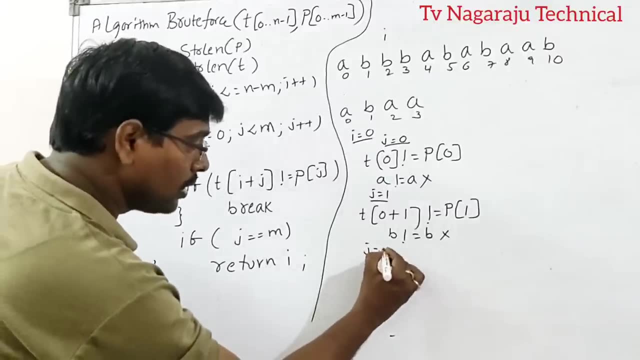 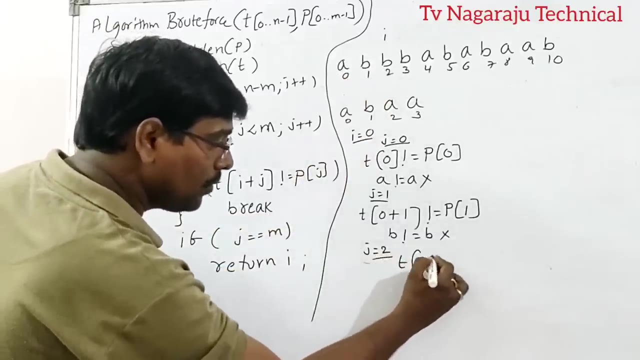 of t1? b Here also b, b not equal to b. Again the condition false. Again the condition false. Now j is equal to 2.. So t of 0 plus 2.. t of 0 plus 2 is not equal to 2.. So j is equal to 2.. 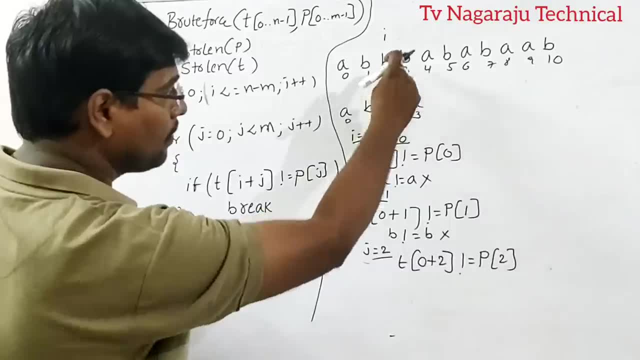 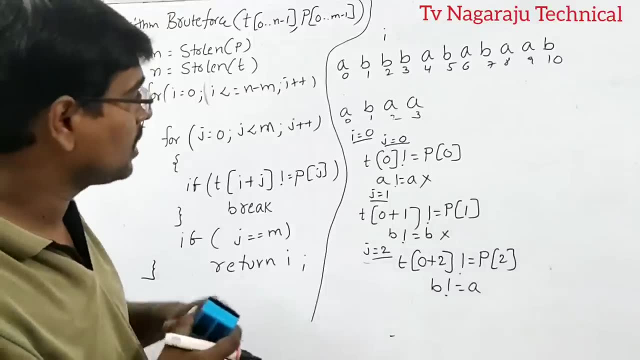 What is 0 plus 2?? b equal to- not equal to a. So we are also doing the same process in the previous example. Yes or no? Compare this one, this one and this one: b not equal to a. Yes. 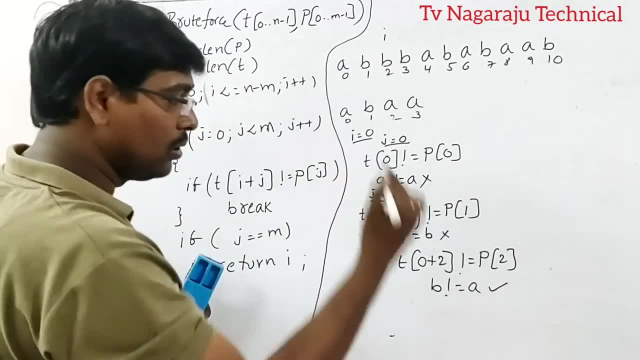 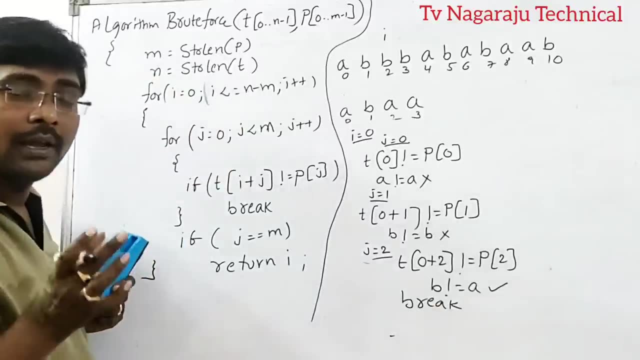 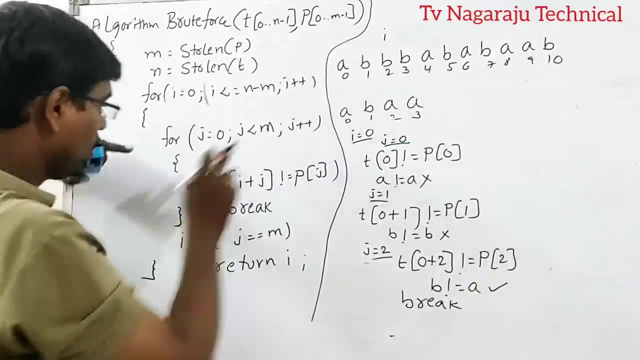 the condition is true, Yes or no, b not equal to a, Then what is applied? If the if condition is true, immediately break is executed. Immediately, break is executed. Whenever the break is executed, we are comparing, remaining one No Comes out of the for loop. 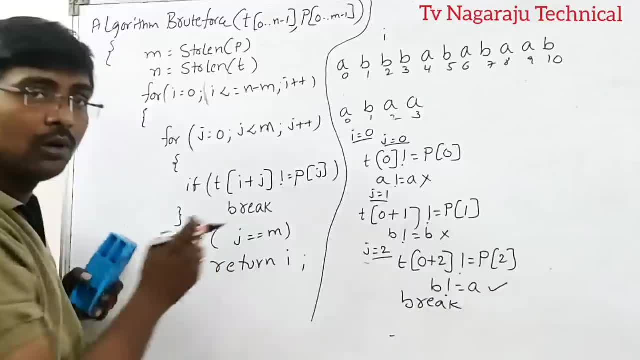 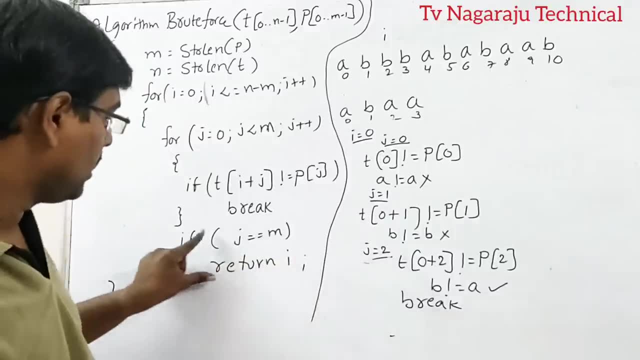 Whenever we are coming out of the for loop, check j equal to, equal to m. What is the value of j? 2. What is the value of m 4. So the condition fail. If is also fail, now move to i plus plus. 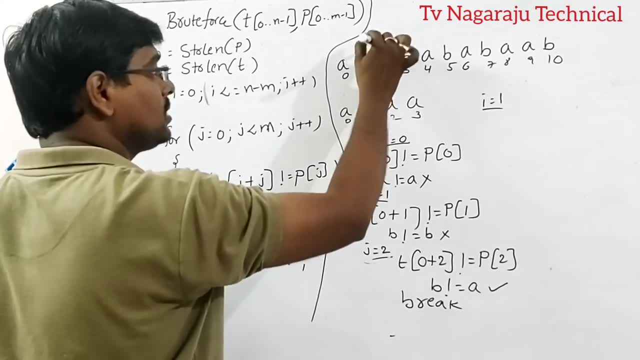 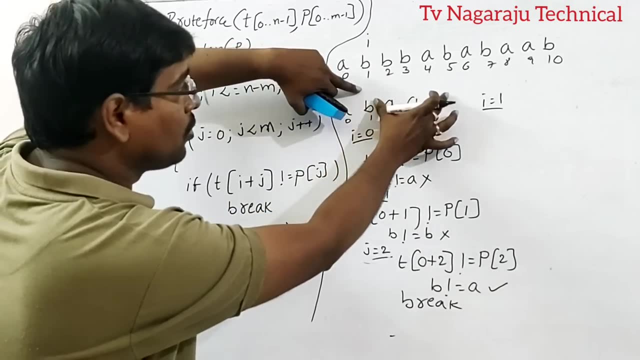 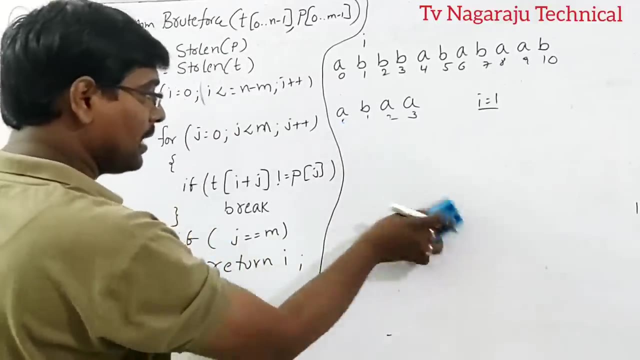 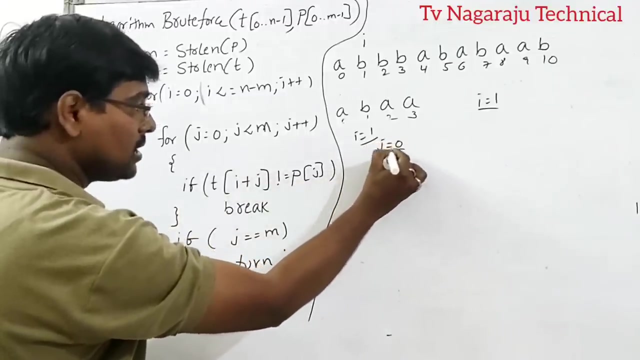 i value becomes 1.. That means now we are again starting this one, Yes or no? So whenever there is a mismatch, this pattern shift to right. Internally, this pattern shift to right. Now explain, for i is equal to 1.. By taking, i is equal to 1, again enter here: j is equal to 0. 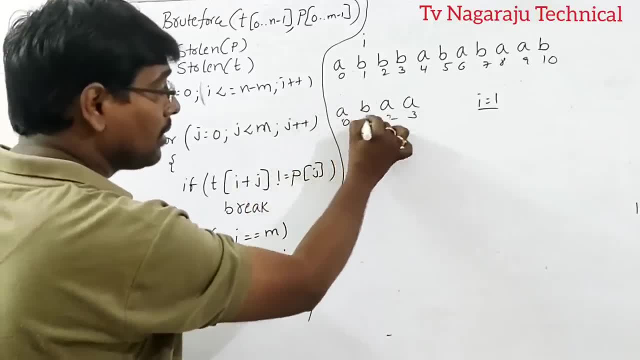 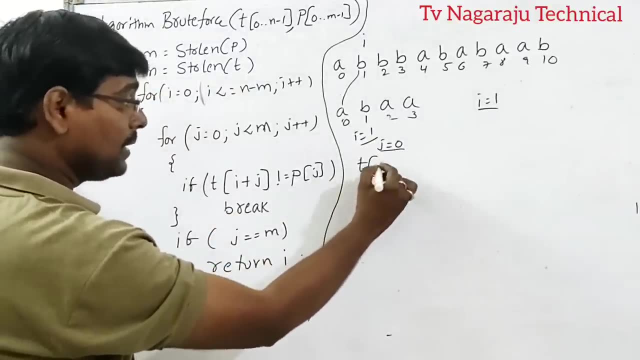 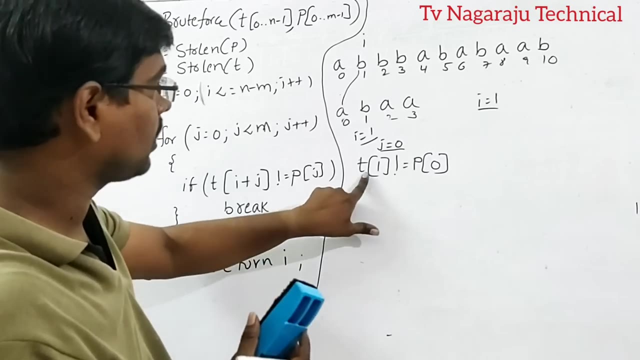 t of 1 plus 0. That means understand the pattern is shifted. We are comparing this one, So t of 1 plus 0 is not equal to p of 0.. Always pattern is taking from the starting, But the i index. 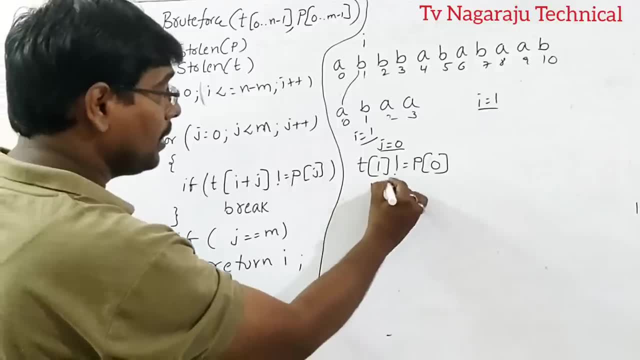 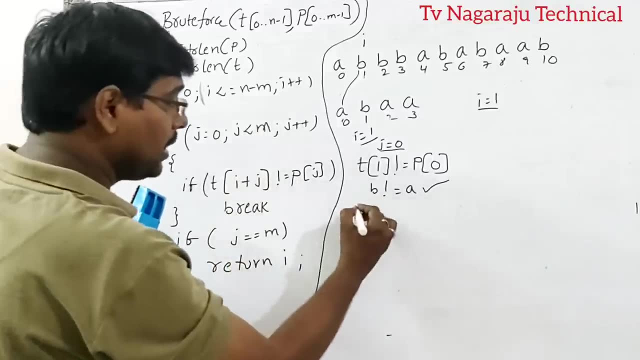 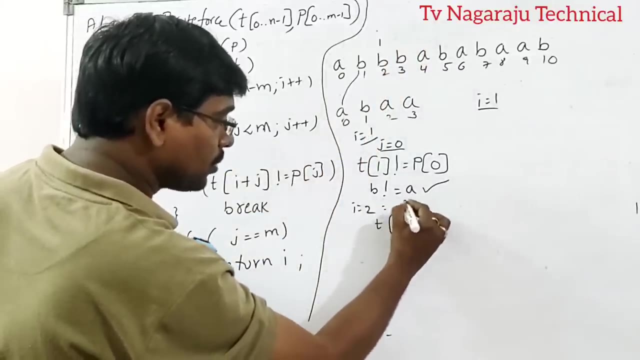 is only changed. Now, what is t of 1? b not equal to a. The condition is true, Break is executed And i is equal to 2.. i moves to this position Again. t of i moves to this position Again. enter inside the loop. 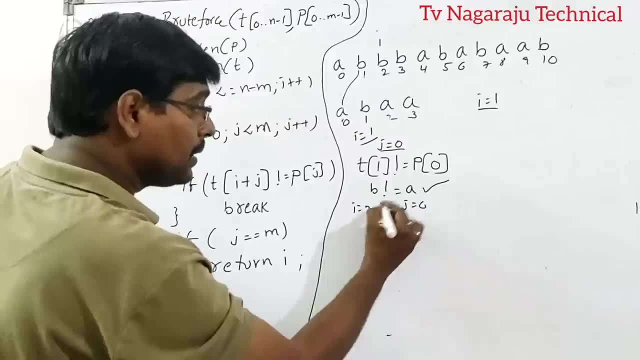 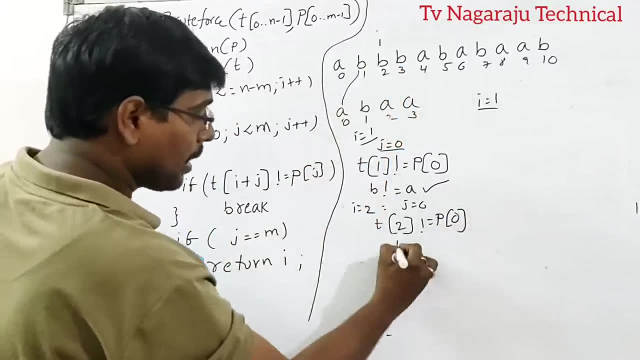 j is equal to 0. So the value of j- is starting with j- is equal to 0.. t of i plus j, 2 plus 0.. Not equal to p of 0. Here, what is the value? b? not equal to a. Again, the condition is true. 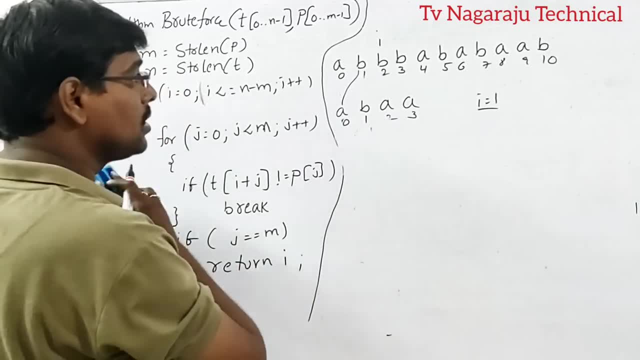 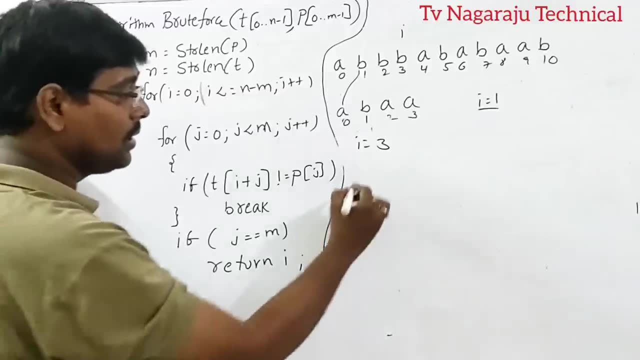 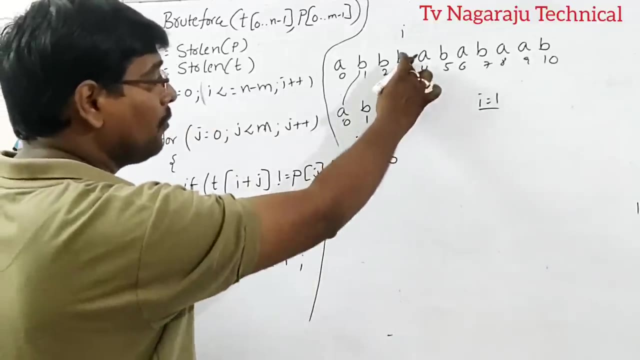 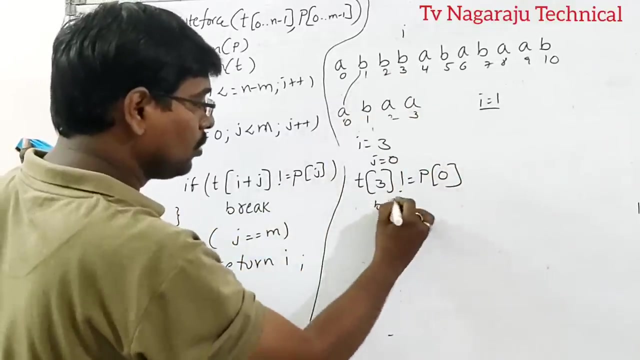 Break is executed. Once the break is executed, i plus plus i value becomes 3.. Right now, i value becomes 3.. j is equal to starting Again enter inside the loop- equal to 0,. p of 3 plus 0 is not equal to p of 0, so b not equal to a. again, the condition is true. 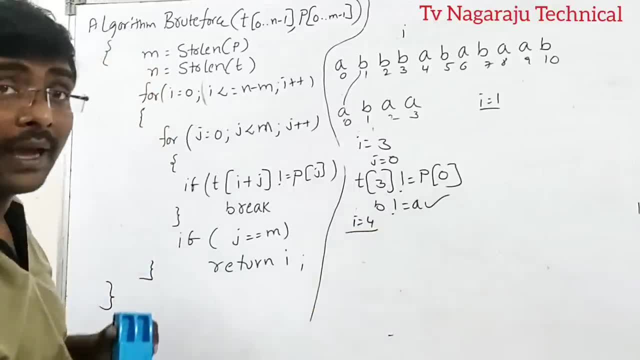 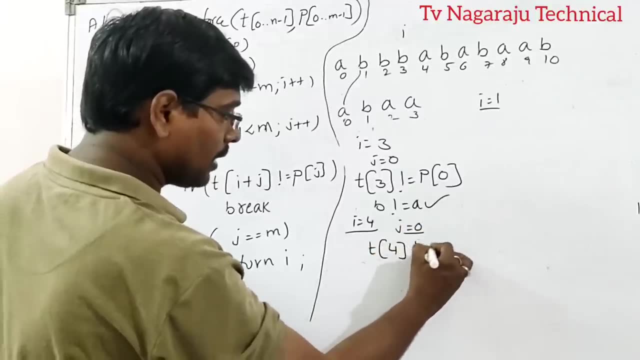 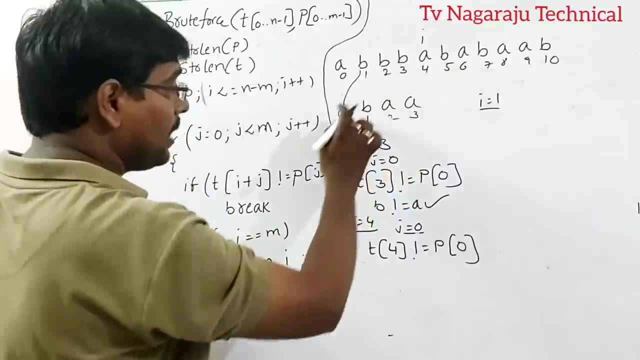 move back. i plus plus i is equal to 4, i is equal to 4,. there j is equal to 0,. p of 4 not equal to p of 0,. 4 plus 0 means 4, t of 4 means this one. a not equal to a condition, false. 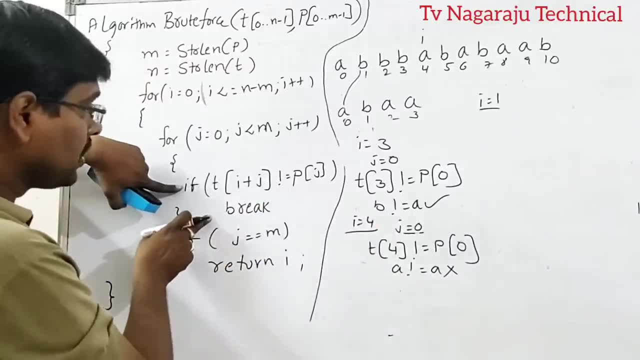 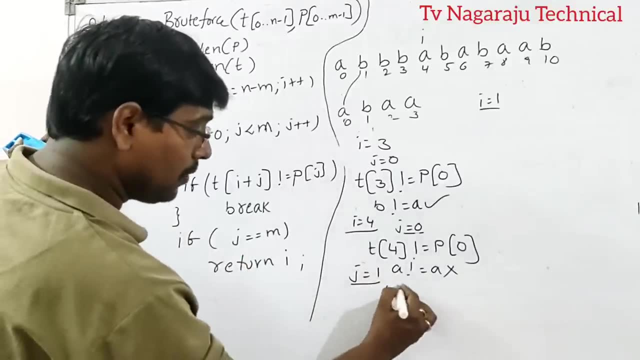 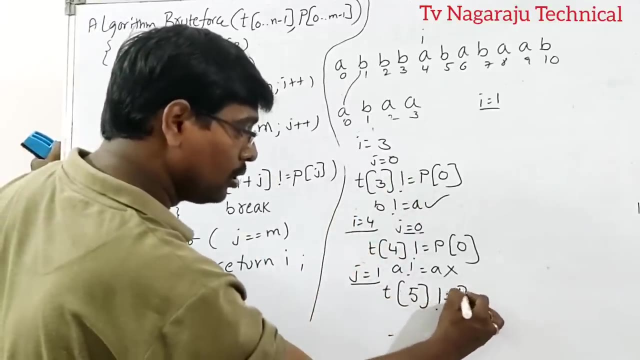 now a not equal to a condition, false. so if is not executed, obviously what happened? j plus plus j value becomes 1, now t of t of i is equal to 4, 4 plus 1, 5, t of 5 not equal to. 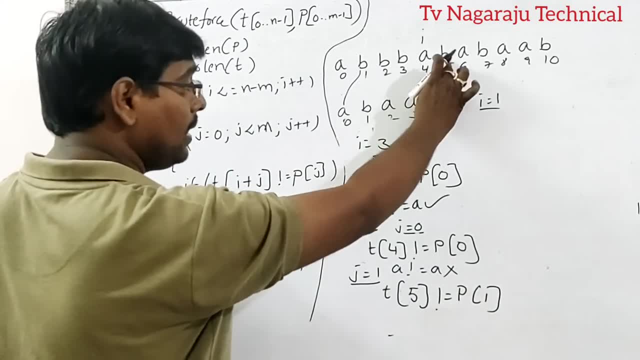 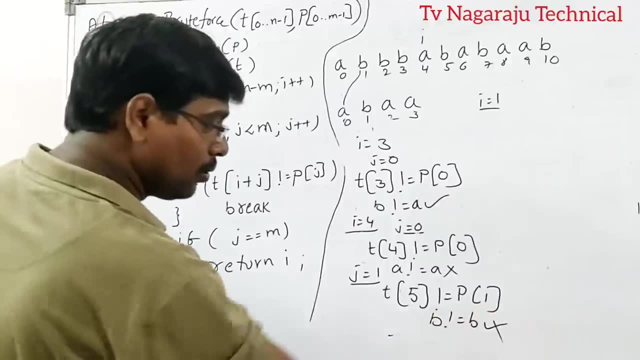 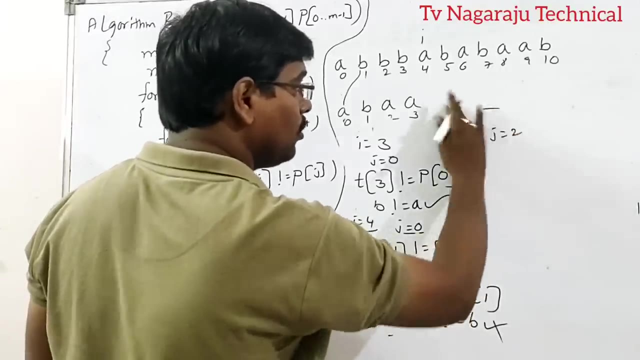 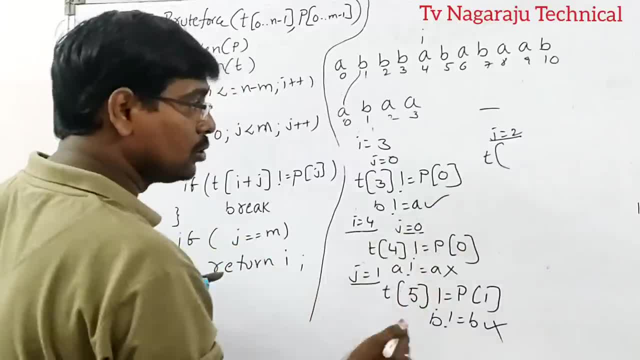 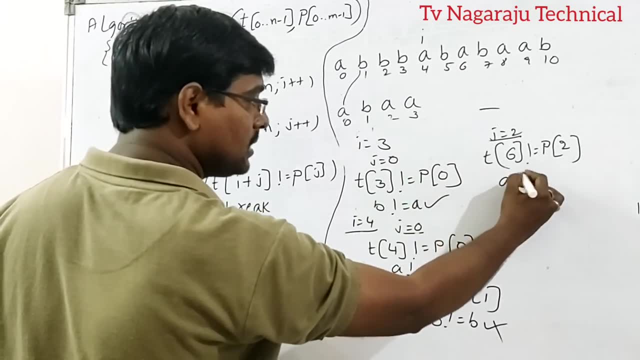 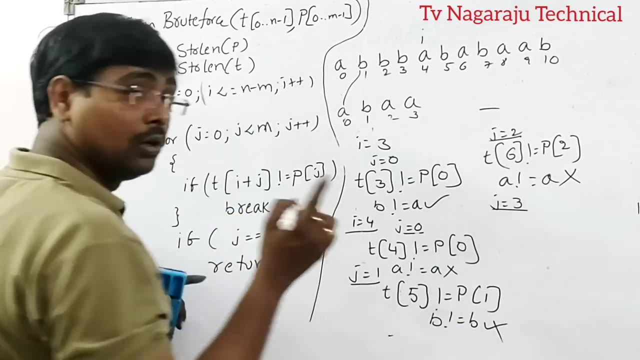 becomes 2, so t of 4 plus 2, 6 is not equal to p of 2,, so t of 6 position, that is a not equal to second position. again, condition: false. Now. now j is equal to 3,, j is equal to 3, t of i plus j. I think you got it. why I written. 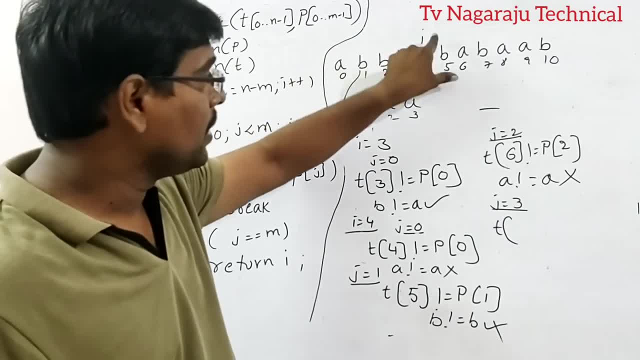 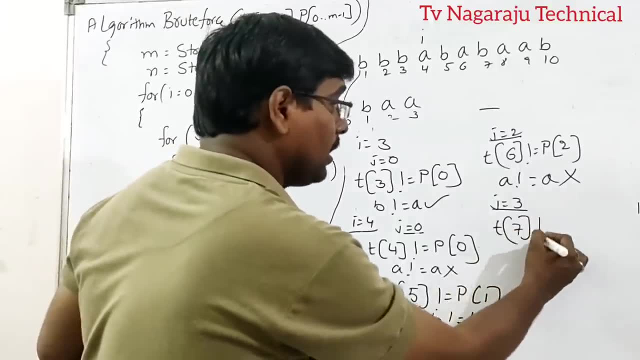 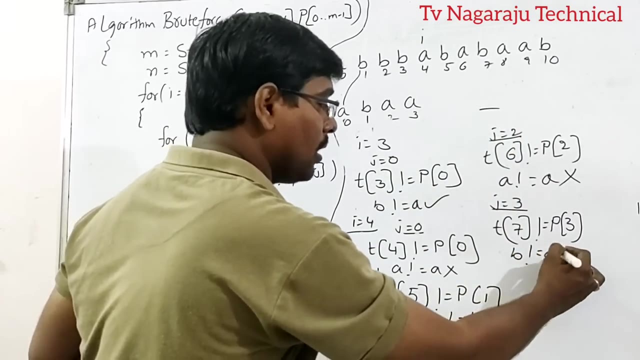 i plus j. first one position is fixed immediately. I am adding 1,, 2,, 3,, 4 until the length of the pattern. so t of 7 is not equal to p of 3, what is t of 7, b is not equal to a, the 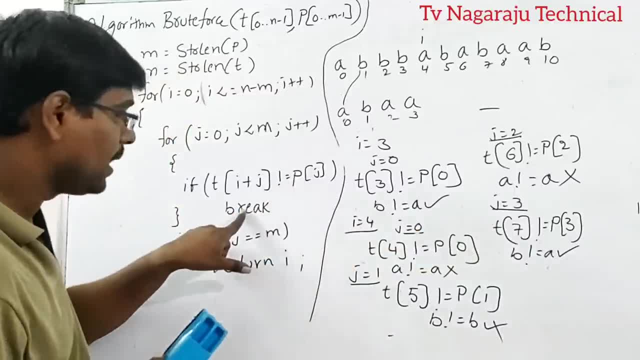 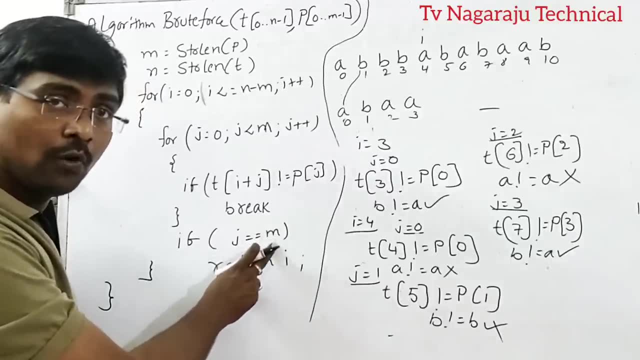 condition: true. Once the condition is true, break is executed. coming out of the break check what is the value of j? 3 is equal to equal to 4, no, so if is not executed, move back. i plus plus. 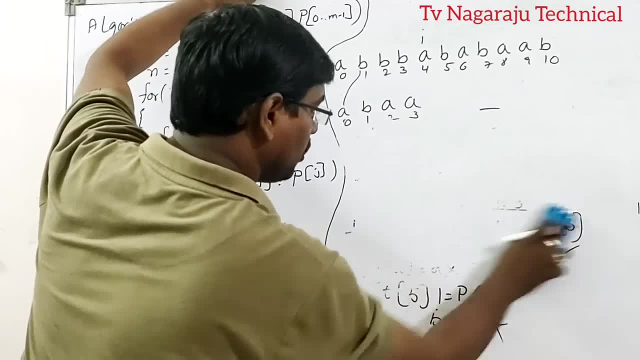 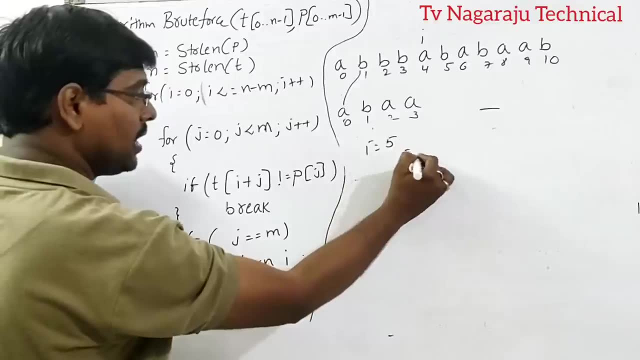 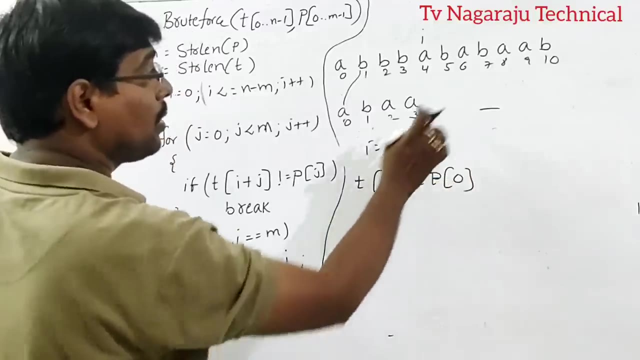 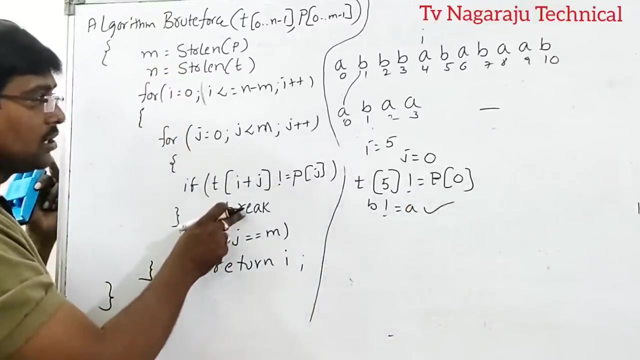 now i value becomes 5, up to i is equal to 4, not happen. now i is equal to 5, again, enter inside: j is equal to 0,. t of 5 not equal to p of 5.. So what is t of 5, b not equal to a? yes, the condition is true, so break is executed. 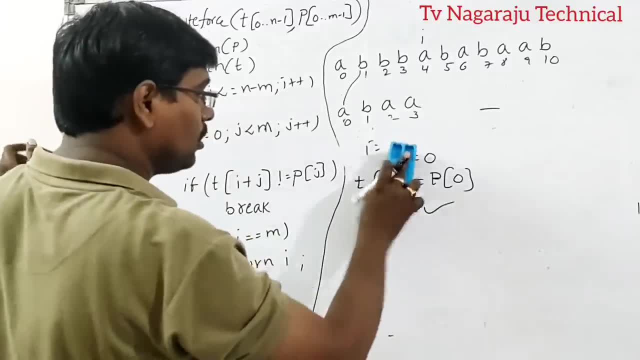 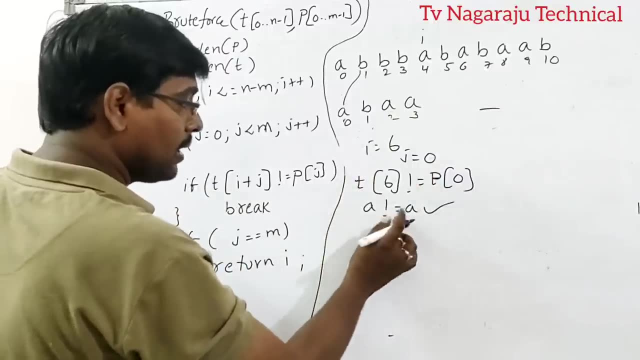 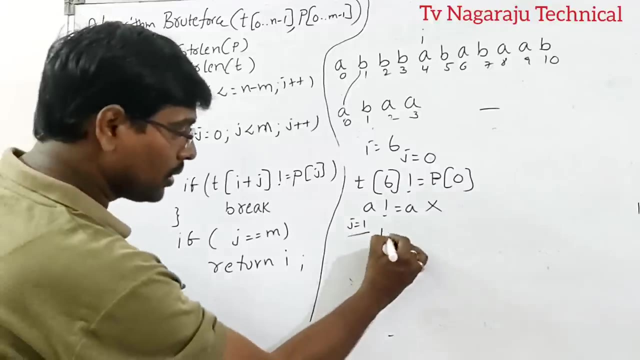 and j condition is also false. again, i is equal to 6,. j is equal to 0, 6,. what is the 6th position? a? a not equal to a. the condition false: j is equal to 1,. j is equal to 1, so 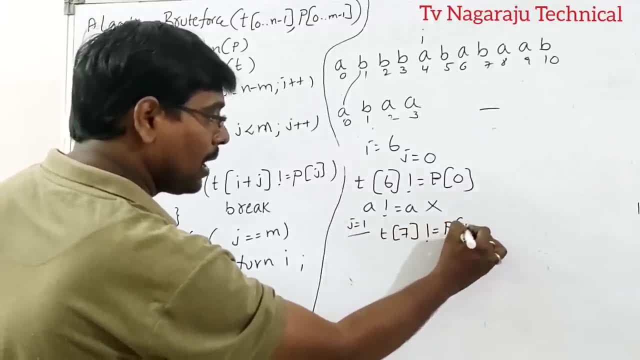 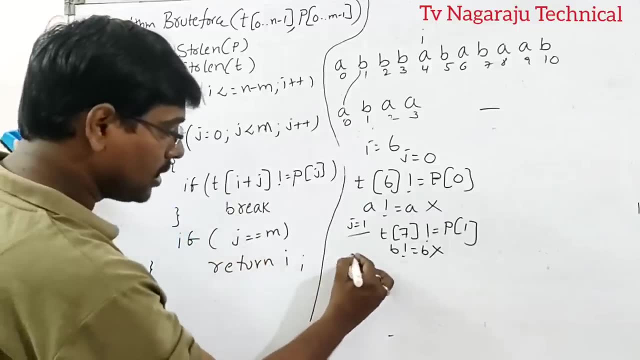 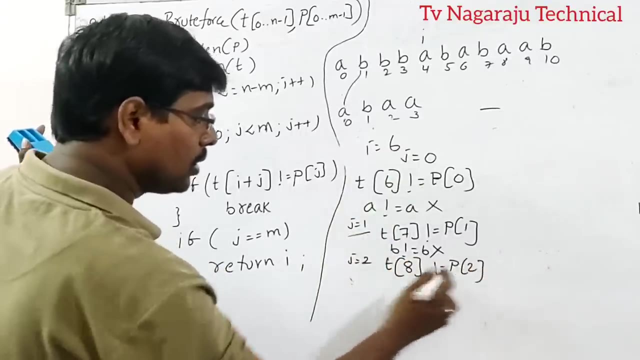 t of 7.. 3 is not equal to p of 1,. what is 7th position? b not equal to b, the condition false. so obviously j is equal to 2.. t of 6 plus 2, 8, not equal to p of 2, so what is t of 8, a? a not equal to a again. 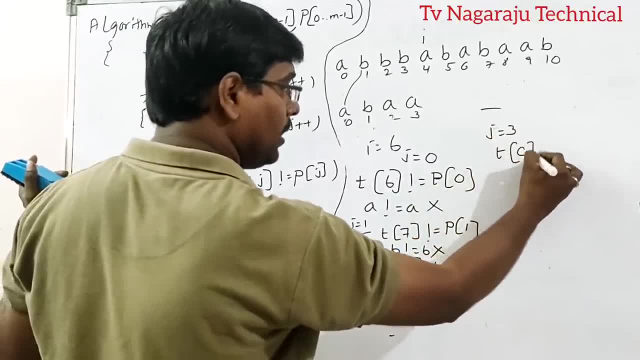 the condition false. Next, j is equal to 3.. t of 9 not equal to p of 3. So t of 9 becomes 8, j is equal to 4, j is equal to 4, j is equal to 3..